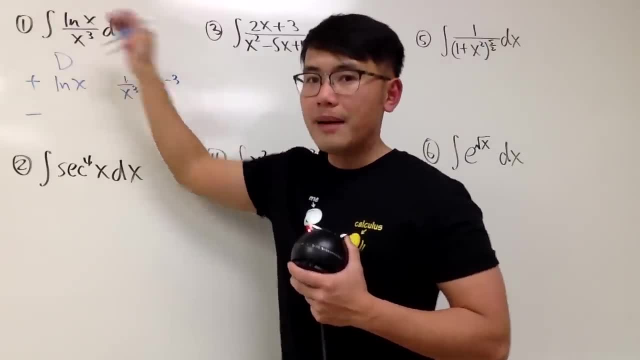 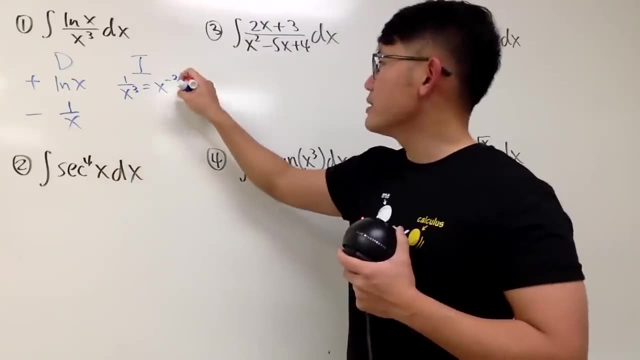 So this is the same x to the negative 3 times natural log of x. Use integration by parts for this And then remember differentiating this. you get 1 over x. Integrating this, add 1, which is going to be negative 2.. 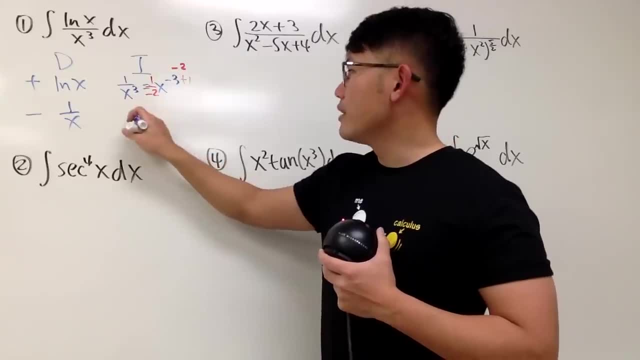 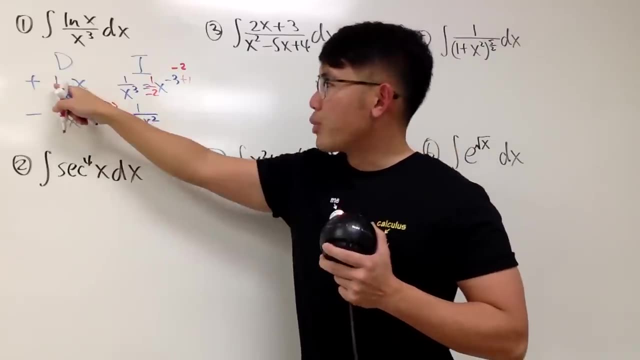 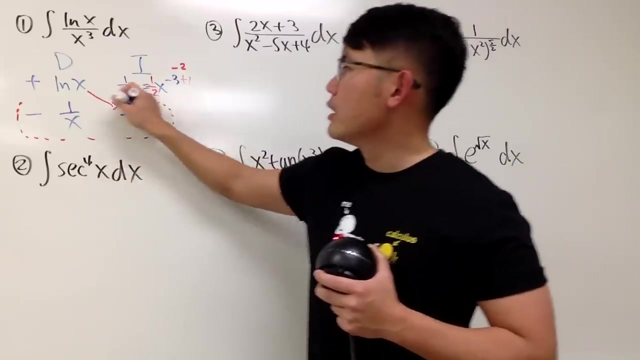 And then divide it by that new power. So we end up with negative 1 over 2 x squared in the denominator. And then, remember, the product of this diagonal is the first part of the answer And then the product of this row you still have to put in the integral. 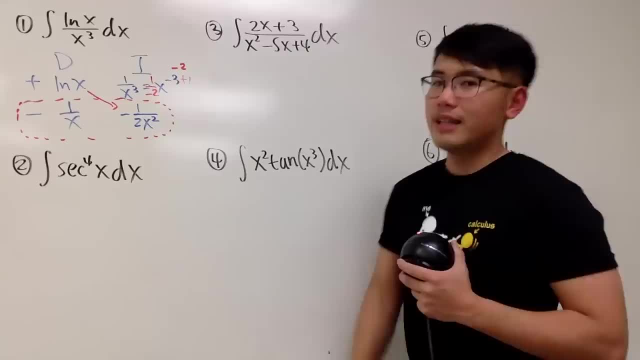 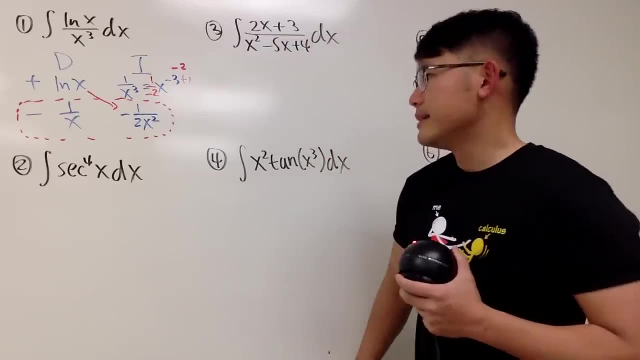 And when you do this times that in fact you can integrate that. So that's the idea. And now let's talk about the next one, the integral secant to the fourth power of x. First of all, you should know some famous ones as well. 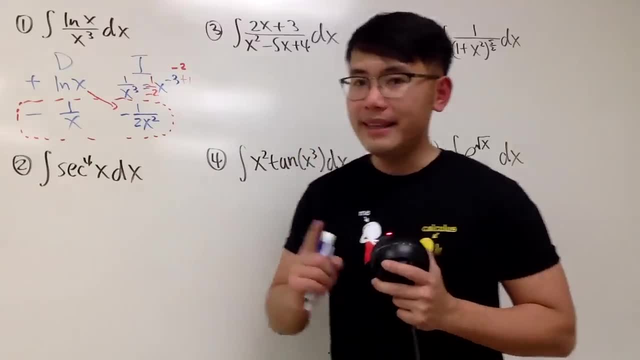 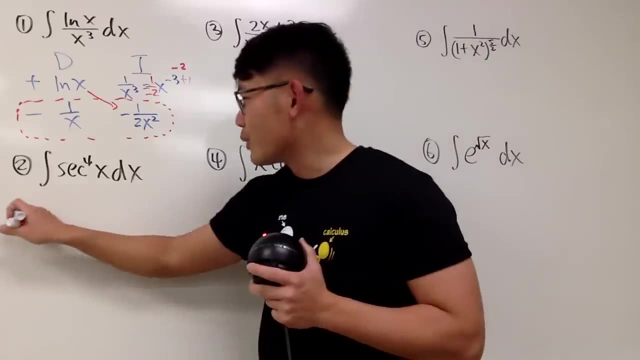 If you have secant to the third power, you have to do that by integration by parts. When you have secant to the fourth power, this is actually much easier. You can just do some trig identities. So I will write this down for you. 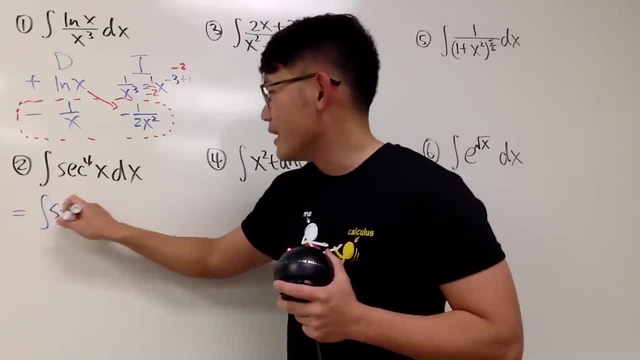 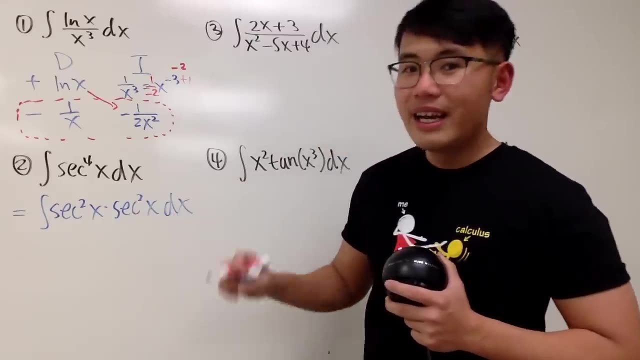 I will actually take out two of the secant. So we have secant squared x right here, and then times, secant squared x right here, And then dx, of course, And then from here I can write secant squared x in terms of tangent. 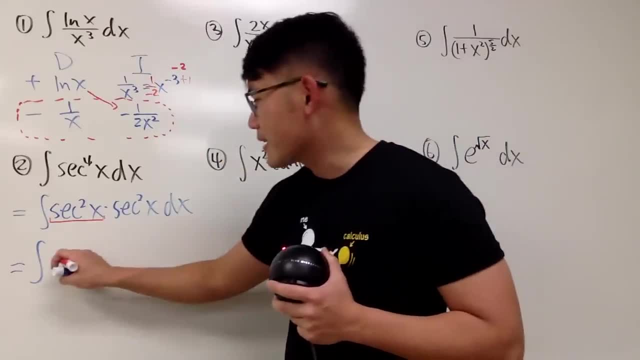 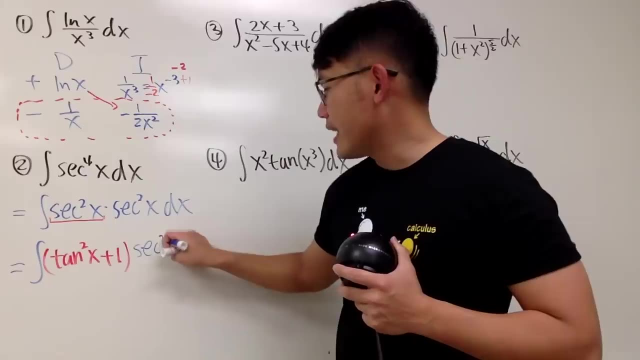 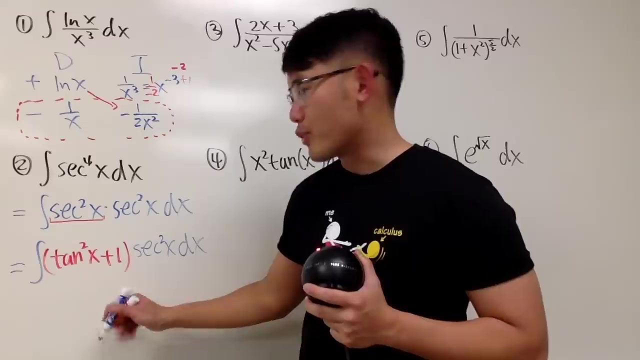 So this is going to give me the integral. This is, in fact, the same as tangent squared x plus 1.. Like this, And then times secant squared x, dx. After this, what do we do? Yes, we can just do a u-sub right here. 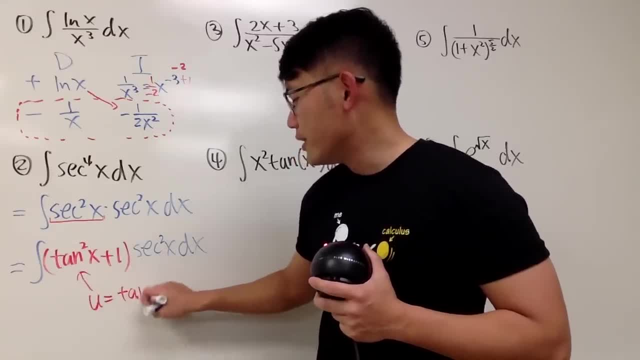 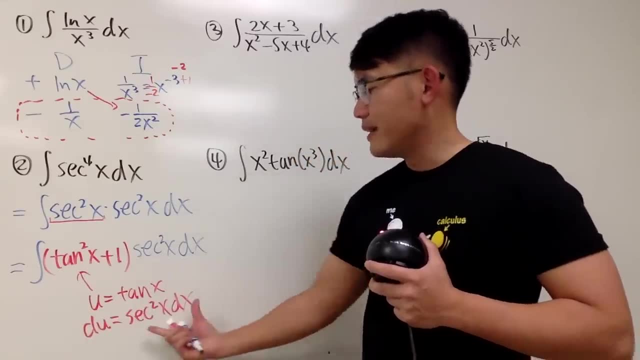 So I'll write this down for you guys: You take u to b, tangent to the first power, x, and then you see du will be secant, squared x, dx. And then you can take this integral to the u-world and you finish it over there. 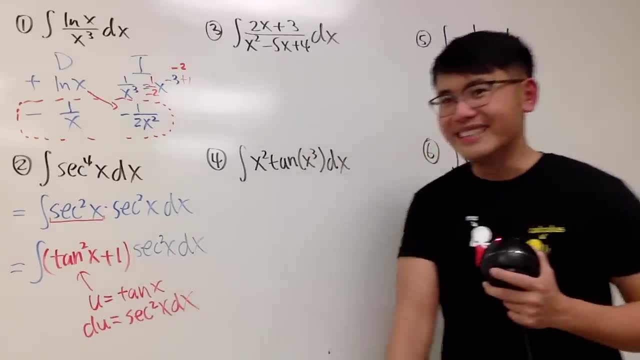 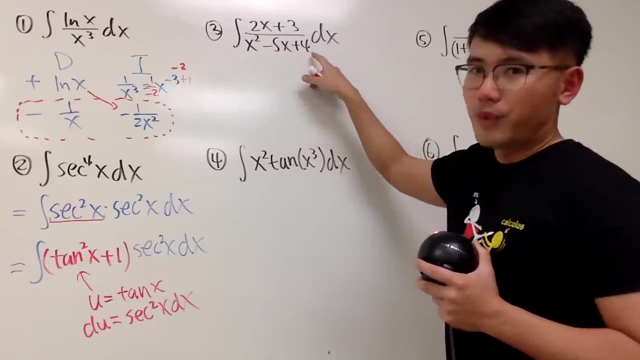 You can be a calculus finisher as well. right Now let's take a look of number 3.. 2x plus 3 over x squared minus 5x plus 4.. First of all, the derivative of the bottom is 2x minus 5.. 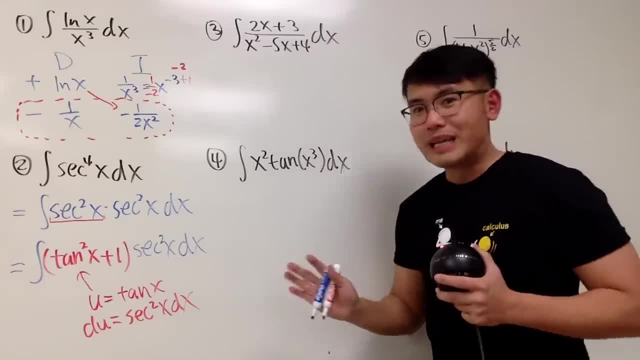 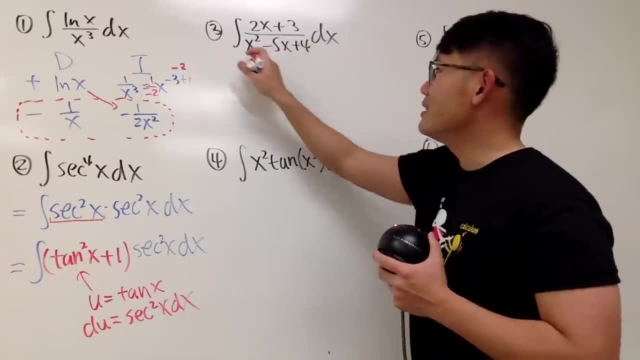 It's not exactly the same. It's the top right. Unfortunately, u-sub doesn't work. This is the rational function On the bottom. we can factor it. So we will just factor this and we can do partial fraction. 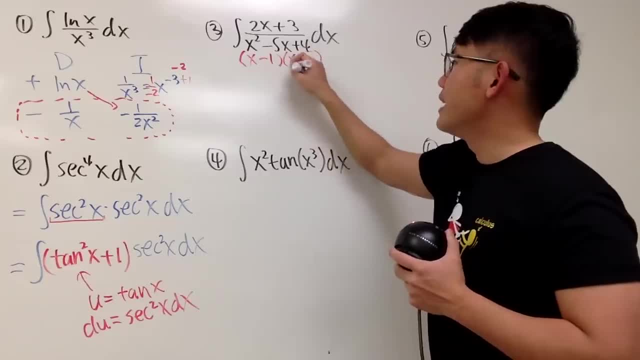 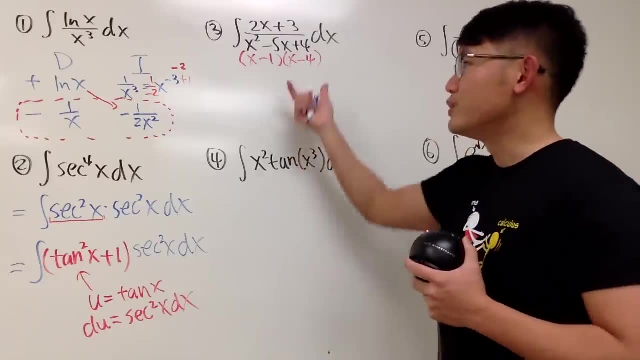 And when you factor this, you get x minus 1 times x minus 4.. And, as you can see, we have two different linear factors. That means we can just do the partial fractions by the cover-up method. So I'll write this down right here for you guys. 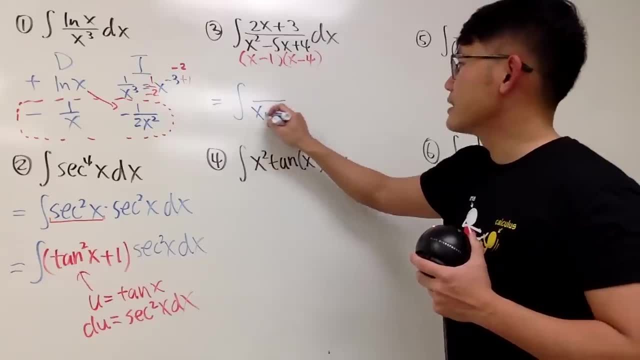 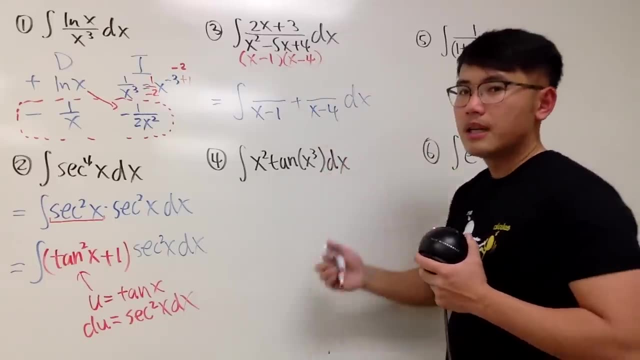 This is the integral, And then the first fraction has x minus 1 as its denominator, And then the second one has x minus 4 as its denominator. To figure this out, this is just going to be a number. You can put down a if you would like. for now, 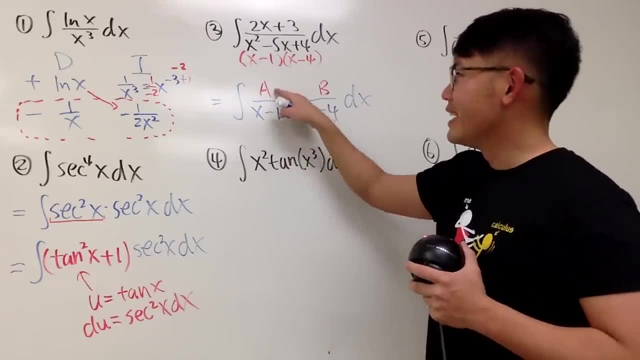 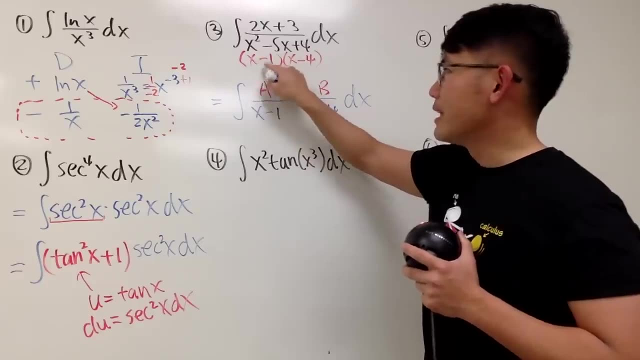 And then this is a b. Now, to figure this out, you go back to the original. You cover the same denominator, which is x minus 1.. And you have to ask yourself: how can you make x minus 1 to be equal to 0?? 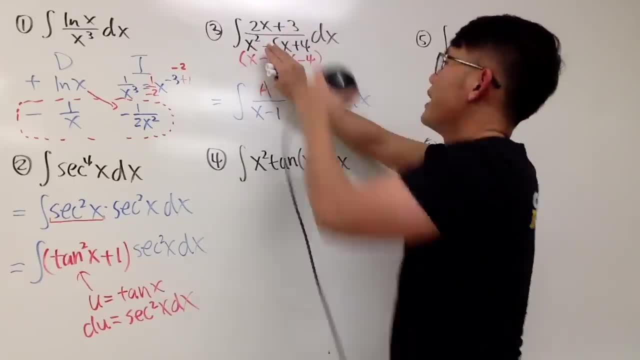 Well, x has to be 1.. Then you plug in 1. And you plug in 1 into the rest of the x On the top. let's do this on your head, OK, 2 times 1 is 2, plus 3 is 5.. 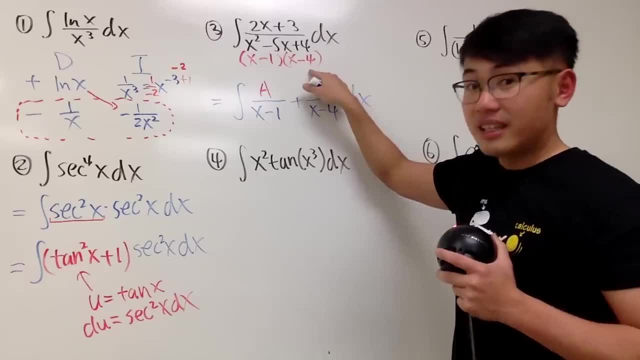 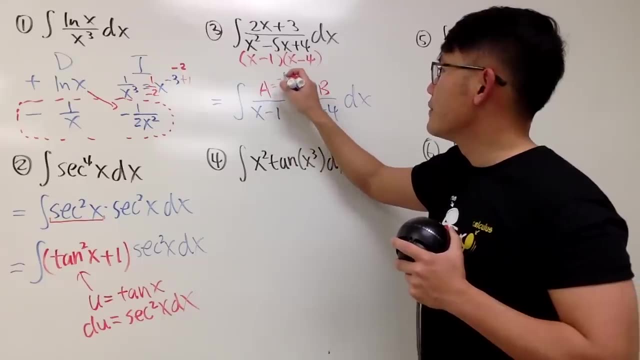 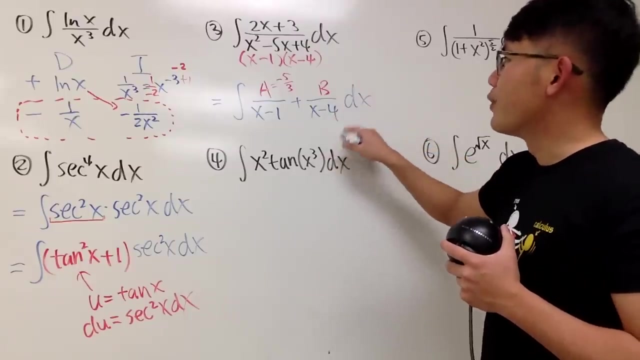 On the bottom: 1 minus 3 is negative 3.. So what does this mean? We end up with 5 over negative 3.. That's 4a negative, 5 over 3,. all right, Now let's do this. b right here: x minus 4 for its denominator. 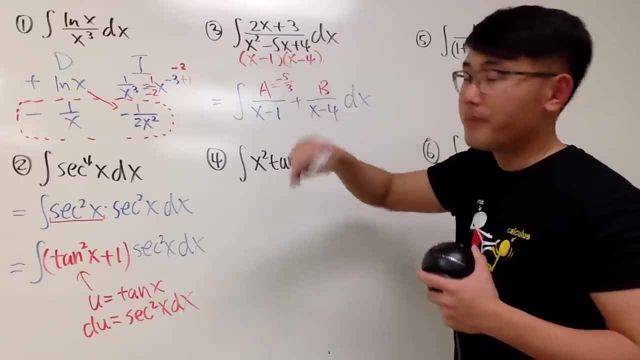 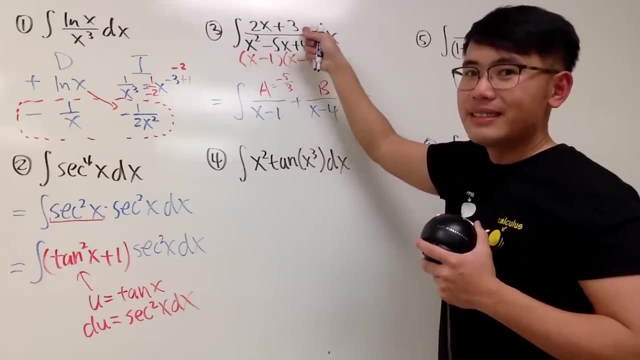 Go back there, cover this up and you have to plug in x equal to 4.. Here and here On the top: 4 times 2, 2 times 4, same thing: 8 plus 3 is 11, divided by 4 minus 1, which is 3.. 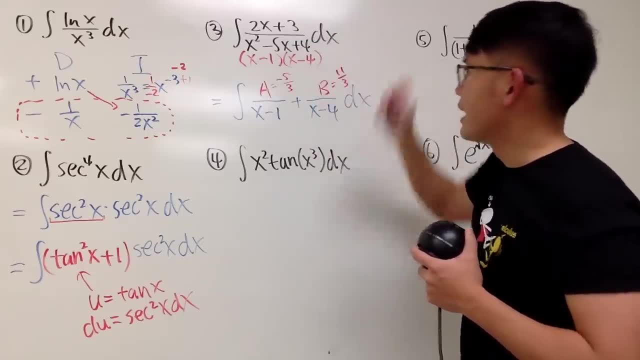 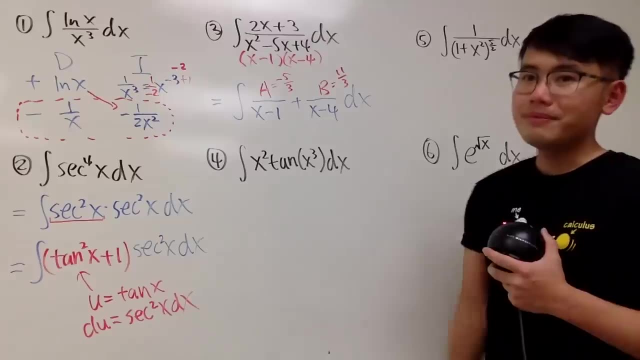 So 11 over 3.. So b is 11 over 3, like this. And then from there you can just integrate this fraction and that fraction, And because this is just x to the first power, you end up with the natural log right. 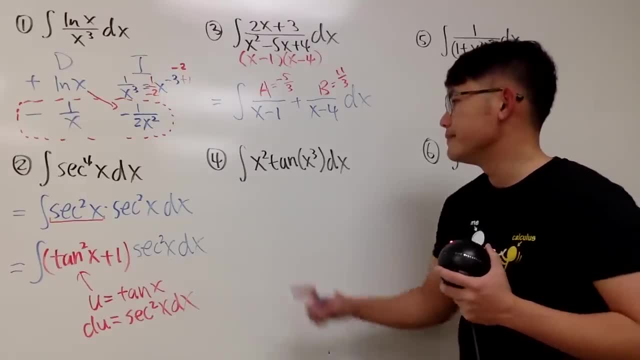 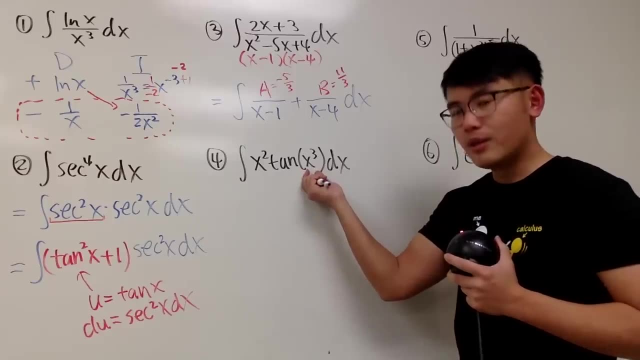 But I'll leave that to you. Now let's take a look right here: The integral of x squared times tangent of x to the third power. What do we do? Take a look of the inside x cubed. When you differentiate x cubed, you get 3x squared. 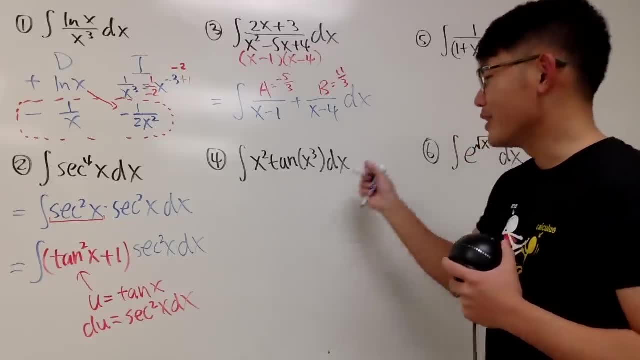 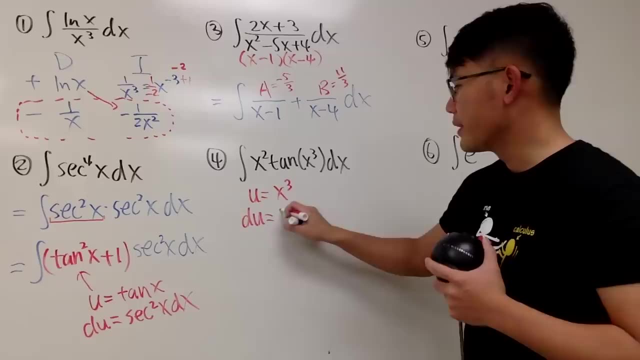 We do have the x squared on the outside. that can help us out. So we can just do this by u sub, Let u equal to x cubed And then from there we get du equal to 3x squared dx. And if you want to isolate the x, I think that will be easier. 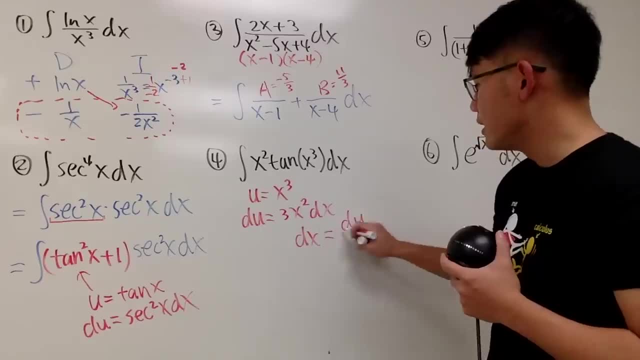 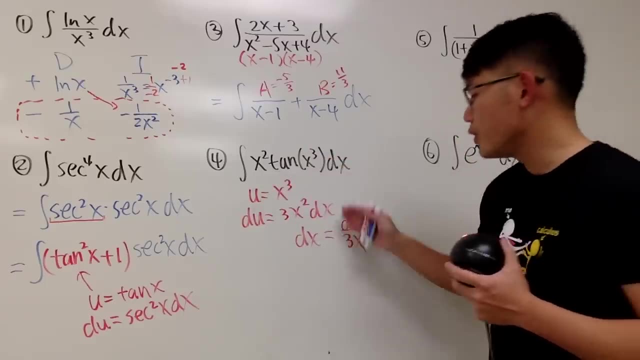 Let's divide this on both sides, We get dx equals du over 3x squared. Put this in the? u world And, as you can see, the x squared will cancel out. You will have one third factor And you will have to know how to integrate tangent of u. 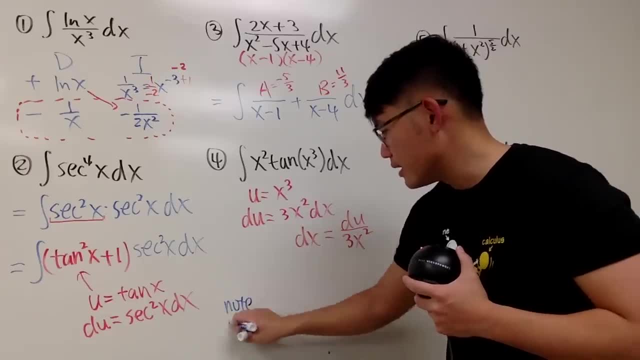 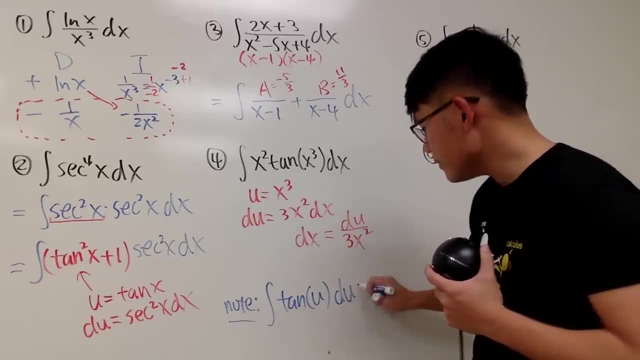 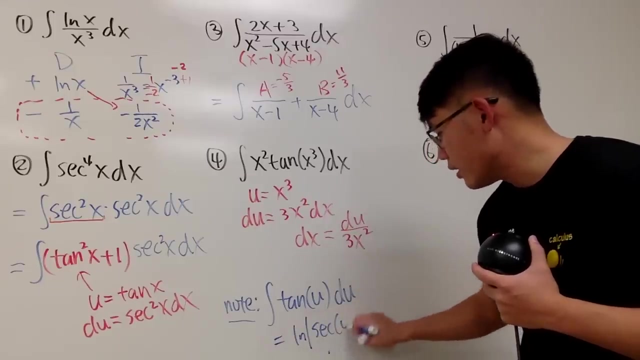 So let me just make a note right here for you guys. You also have to remember that the integral of tangent- And let me just put down u for this for you guys, This right here, is equal to the natural log absolute value of secat of u and then plus c. 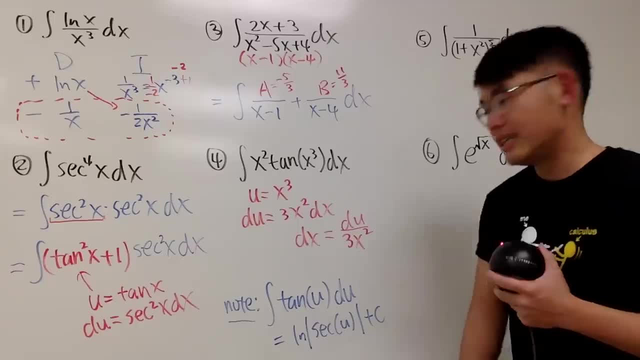 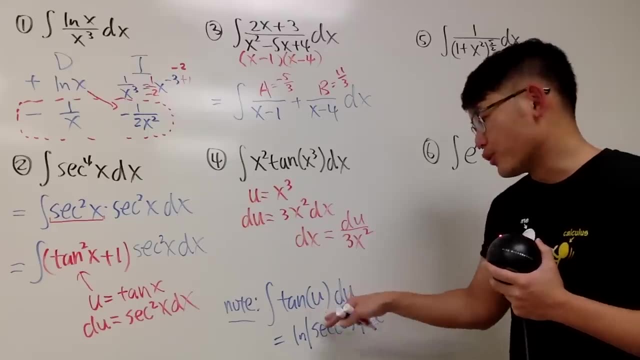 You have to know this so that later on you can just use this. And of course, to integrate this, you can write this as sine over cosine And then do another substitution. But you use u already, so you can use w and all that. 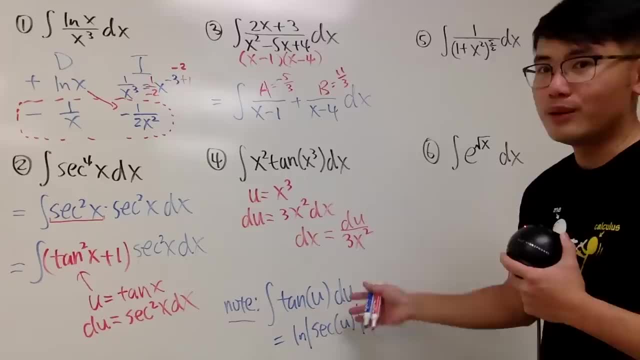 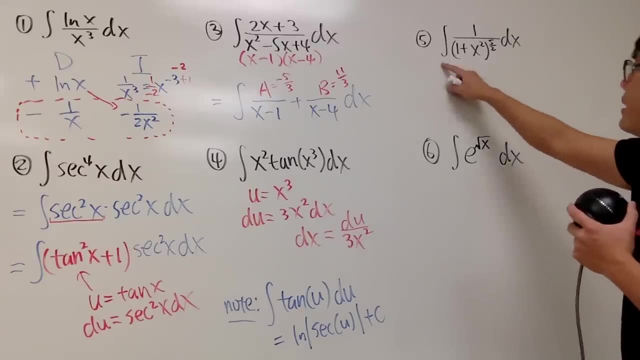 And you do have the one third factor, But you know I'm not working that out, That's your job, right? So you have to remember this, so you can finish that. Now let's take a look at this. We have the integral of 1 over 1 plus x squared. 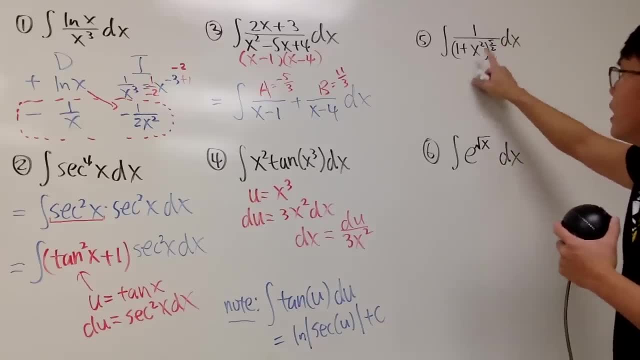 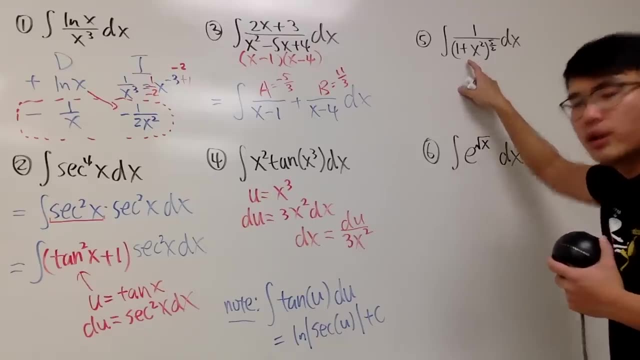 And then to the 5 over 2 power. Well, this is so intimidating, But inside here we have two terms: 1 plus x squared, And we have to know that It's just like this. Look at that: 1 plus tangent squared. 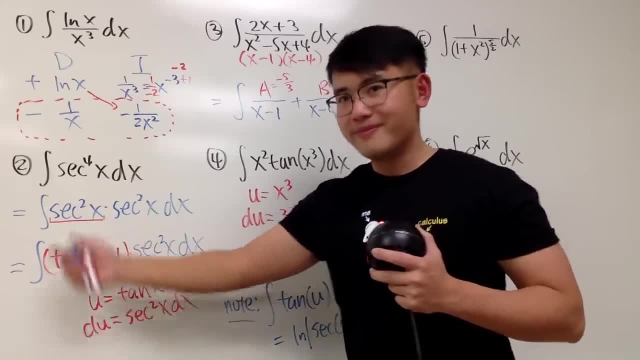 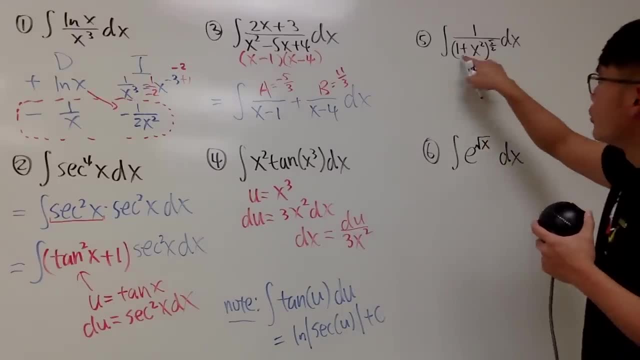 This right here is equal to secant squared. It's just one term. You can put this right here. Yes, we'll just do a trick. stop for this one. So when you have a number squared plus x squared, we'll take x to be tangent. 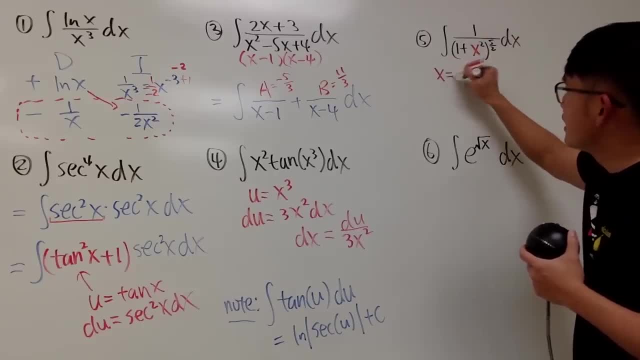 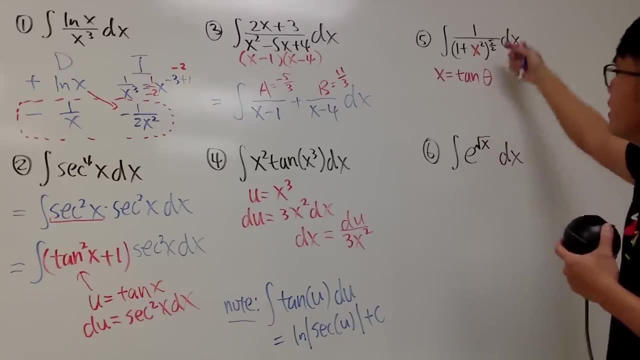 You let this x to be tangent, Take x to be tangent And we take this to the theta world. And you really have to do tricks up here, because on the top it's just a 1. If you have x, you can just do a regular use up, right. 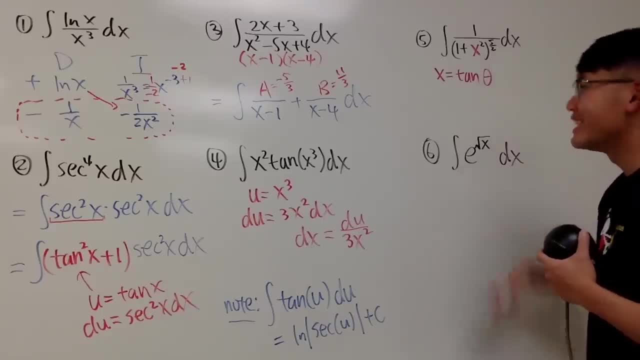 You can just let u equal to this, But unfortunately we don't have that. Take x to be tangent theta. And don't forget dx is equal to secant squared theta, d theta. You have to remember to put this Back for dx. 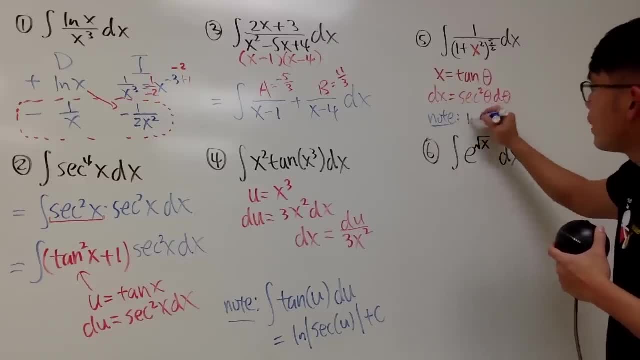 And then you also have to know that when you have 1 plus tangent squared theta, this gives you secant squared theta. Yes, it's kind of weird, because the derivative of this is secant squared And then 1 plus tangent squared is also secant squared. 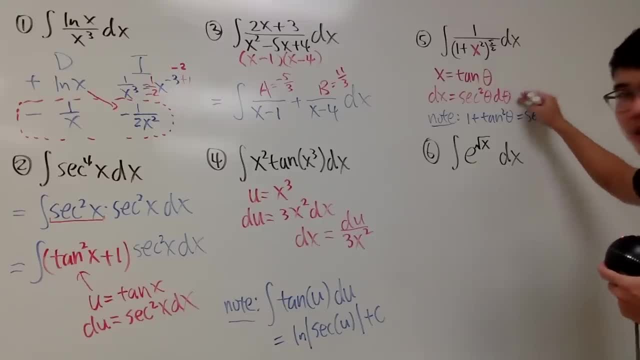 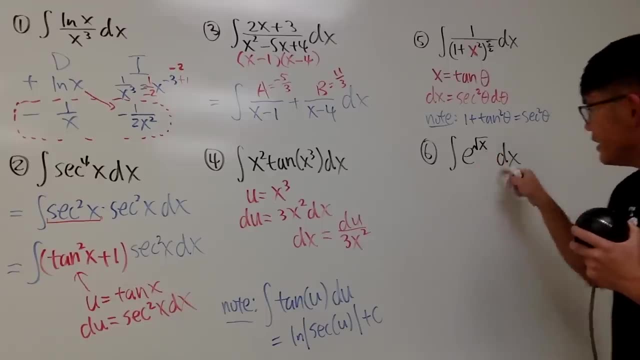 But this is a trig identity. This is the calculus derivative. right here, right? So now let's take a look at the integral of e to the square root of x. This, right here, seems kind of weird. It's kind of impossible, right? 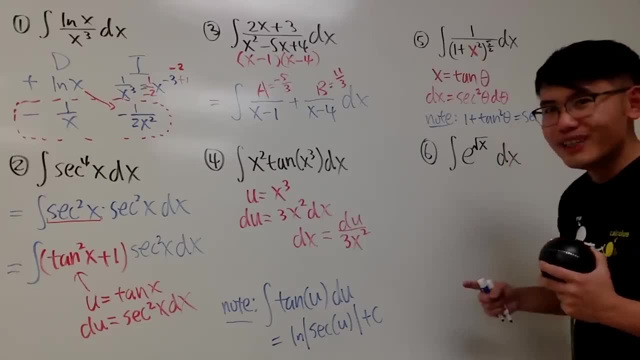 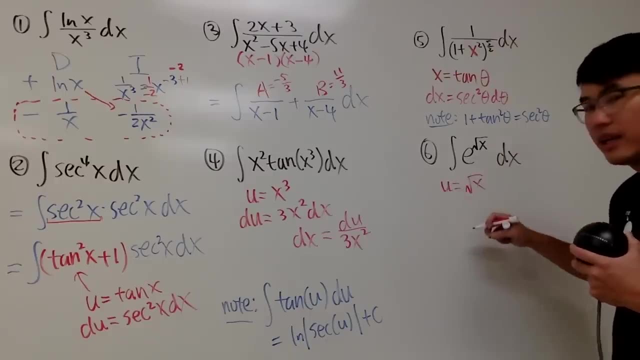 But the truth is, if we take this integral to the? u world, you will see what we need to do. So let's make that happen. I will first let u equal to this, namely square root of x, And then, before you differentiate both sides, 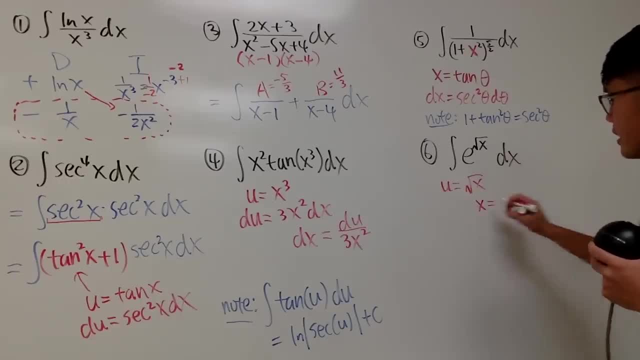 well, let me just square both sides so I can get x equals to u squared, Because this way I can just look at this and differentiate both sides. I get dx that's equal to 2u du, And then I can just take this integral to the? u world. 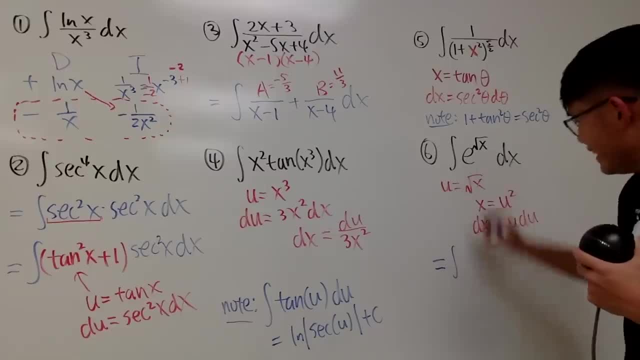 and then you will see that we will have the integral of e- This is my u now- and then times the dx is 2u, du, like this, And then, as you can see here, we have 2u to the first power, times, e to the u. 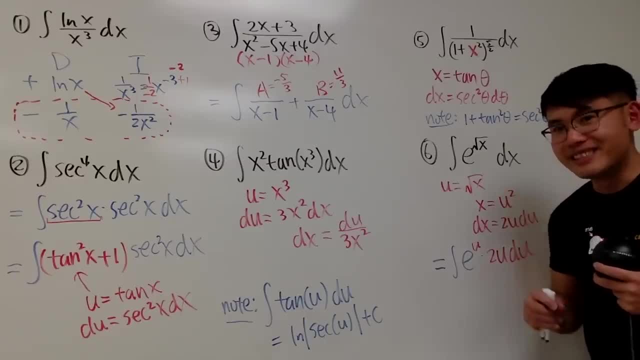 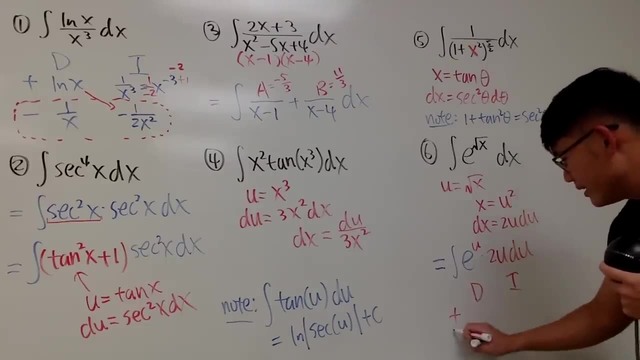 And yes, in this case you can just do the DI method, namely integration by parts. So you're going to do the DI setup right here and in this case we can actually finish the derivative. so I'll put on 2u right here. 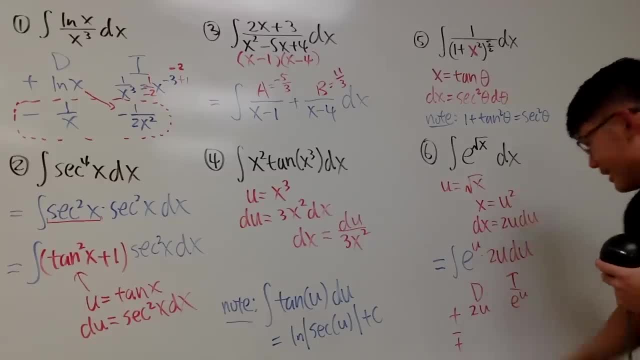 and then we'll integrate e to the u and then, differentiating 2u, you get 2. differentiating 2, you get 0. so you stop right. that's the first stop. when you see the 0 in the d column and, as you can see, 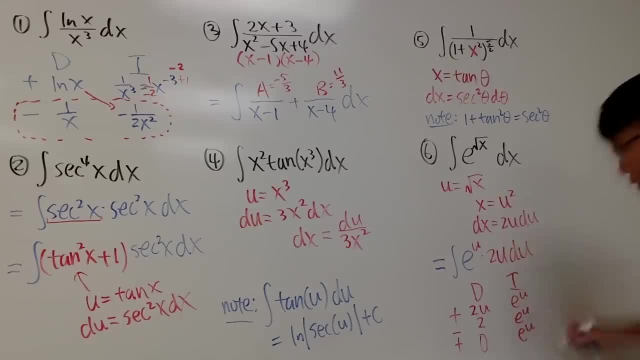 when you integrate e to the? u, you always get e to the? u. so this is pretty much it, and then, of course, the product of the diagonals, along with the sign in front. they will be the answer. however, once you finish that, be sure you go back to the x. 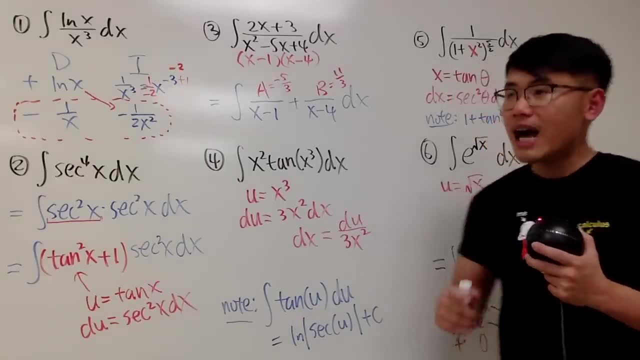 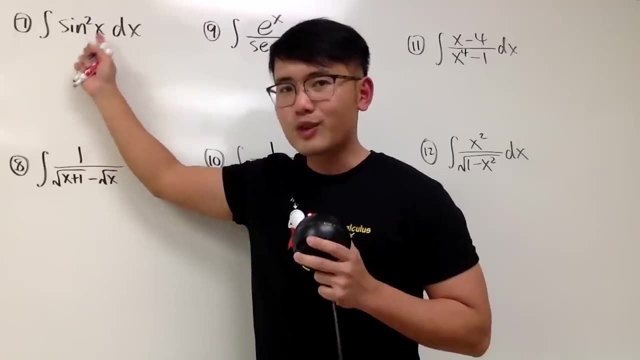 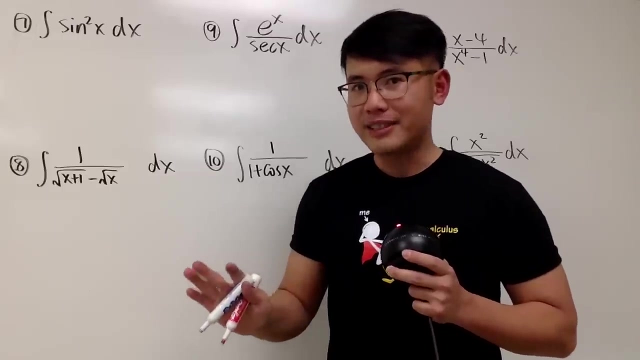 world, and of course I will leave that to you guys. and now let's take a look of the other questions right here, okay, number 7: integrating sine square x. well, in this case, as you can see, we don't have cosine x to help us out, so don't do use up yet. 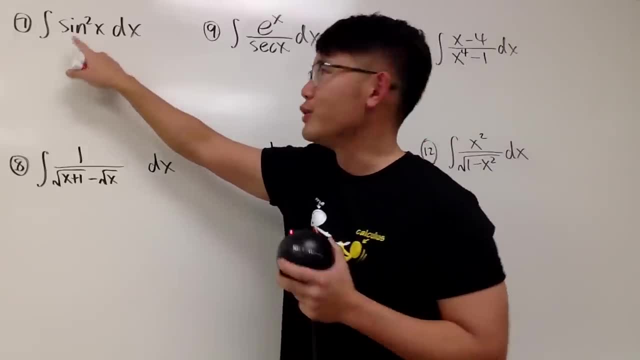 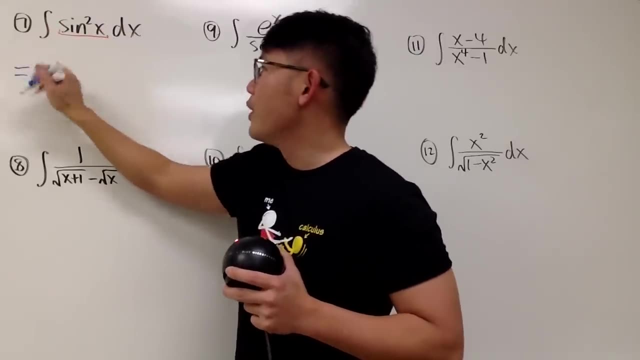 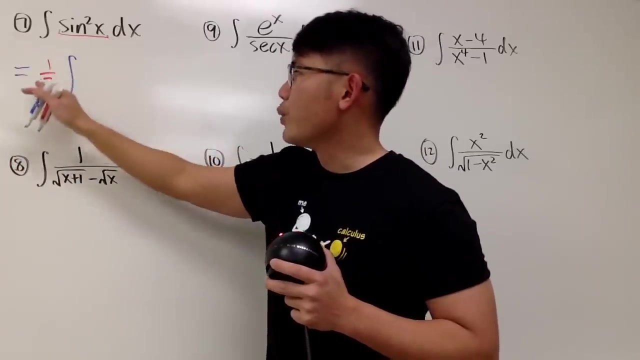 in this case we have to actually use the identity to reduce the power. when we have sine square x- we know this right here- is equal to one half, which is the constant multiple. we can take that to the front of the integration and then the integral. again this is equal to one half. 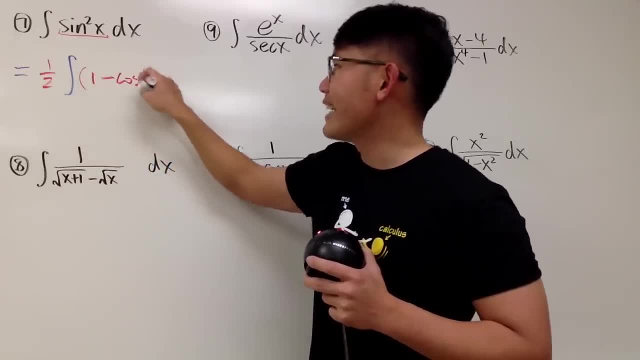 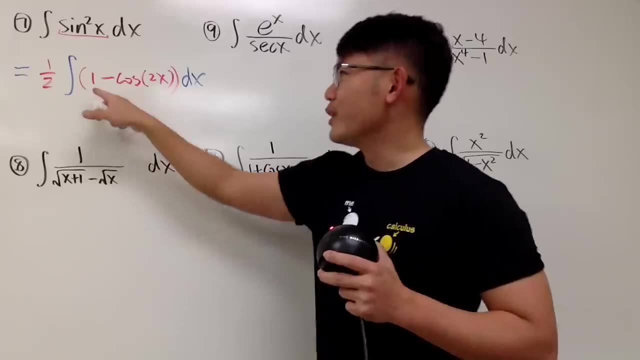 times 1 minus cosine of 2x, like this, and you have the dx and then right here you can just go ahead and integrate, integrating 1 in the x world and also integrating this in the x world, and right here you have to do a use up. but I will leave. 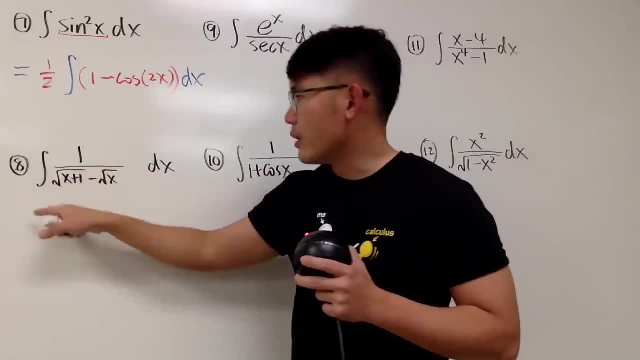 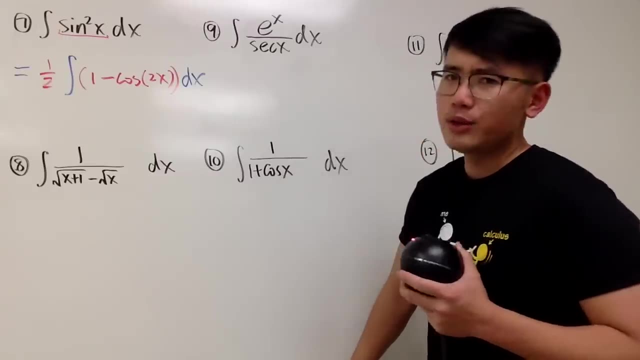 that to you guys. now number 8: the integral of 1 over square root of x plus 1 minus square root of x. hmm, in this case, I don't think use up can help us out of 2 square roots. I don't think use up. 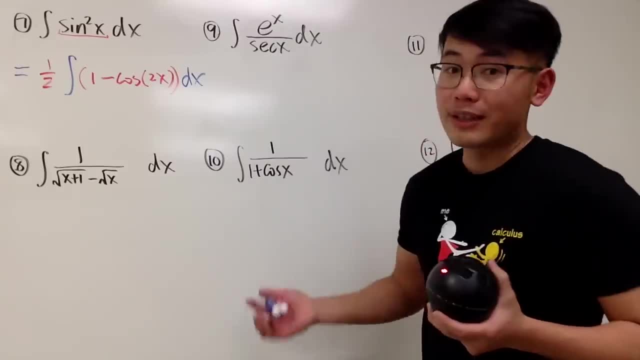 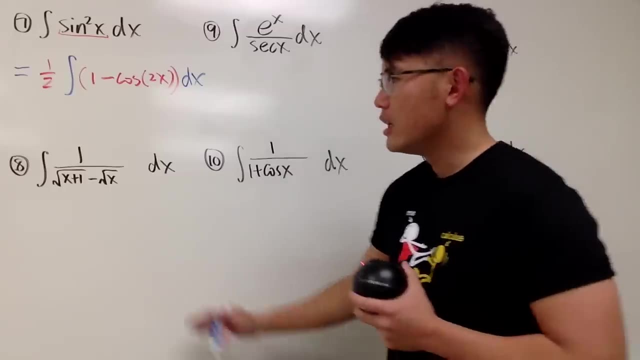 can work this out nicely for us. it maybe works, I don't know, but I know that maybe I can get rid of the square roots in the denominator, just like the Google days. right, we can multiply the bottom and the top by the conjugate, so we can say bye, bye to the. 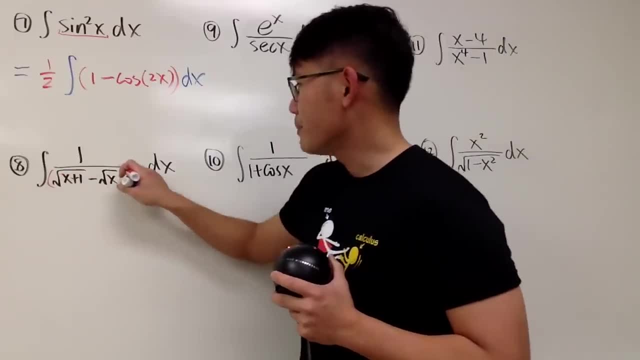 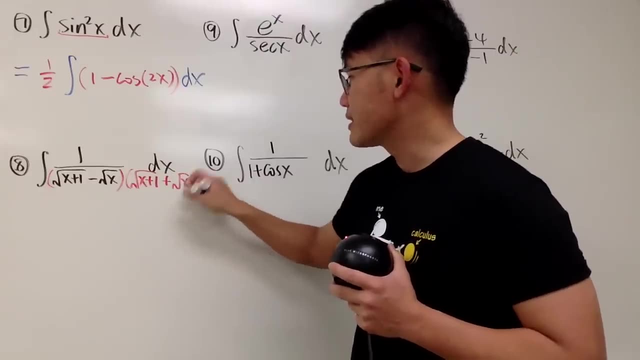 square root in the denominator. so let's do that. let's multiply the bottom by square root of x plus 1 and change the minus to a plus, and then you have the square root of x. and of course, do the same on the top square root of x. 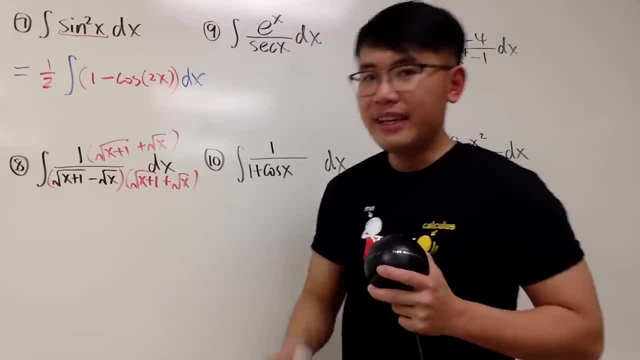 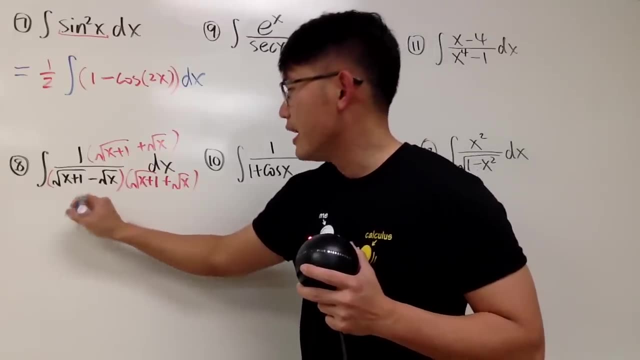 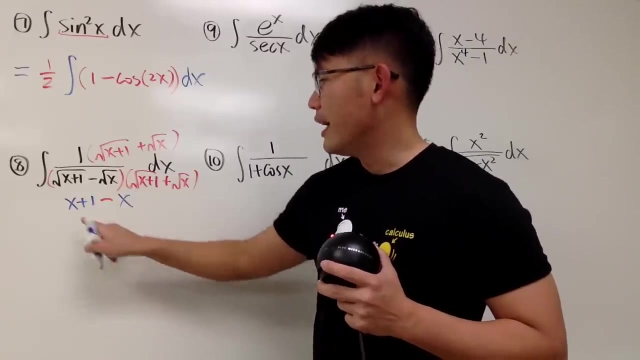 plus 1, plus square root of x. and the beauty of this is that when you multiply this and that, remember- we end up with this thing square, which is just x plus 1, and then minus this square, which is just x. and you see, x minus x is just. 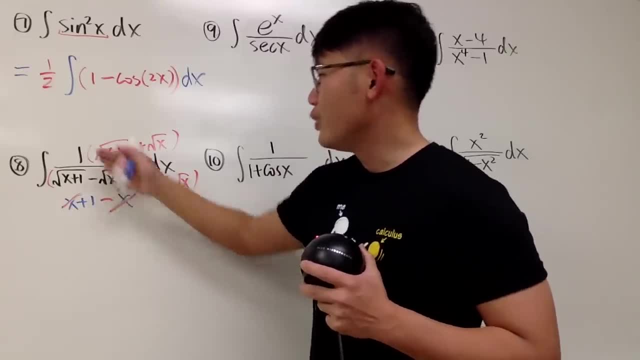 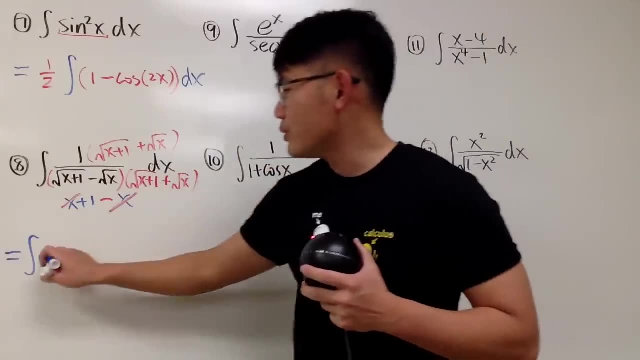 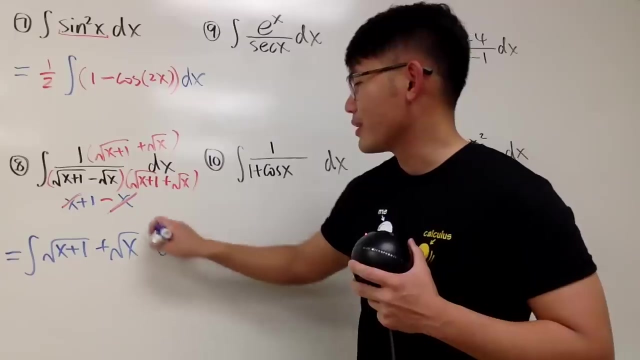 gone. and then of course, we have the plus 1 and you have this over 1. of course the over 1 doesn't matter. in another word, we are just integrating square root of x plus 1 and then plus square root of x, like this, and then put down the dx right here. 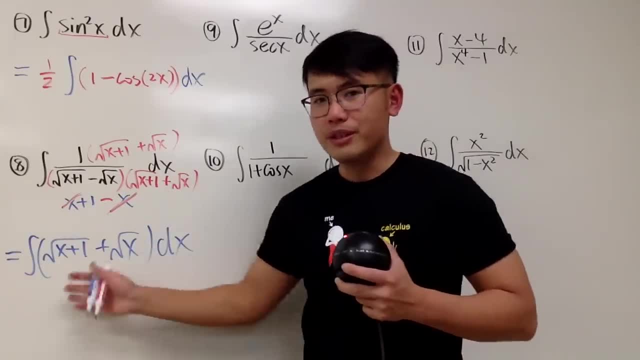 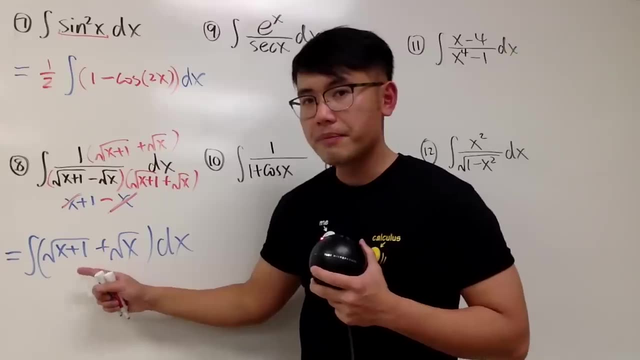 and you can put parentheses right here. be sure you just integrate this and maybe you can do a little bit use up stuff, because there are schools in this institution but the inside here is just x. the derivative of this is just 1, so if u equal to 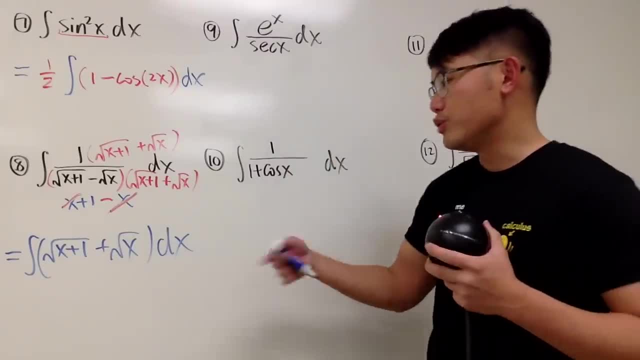 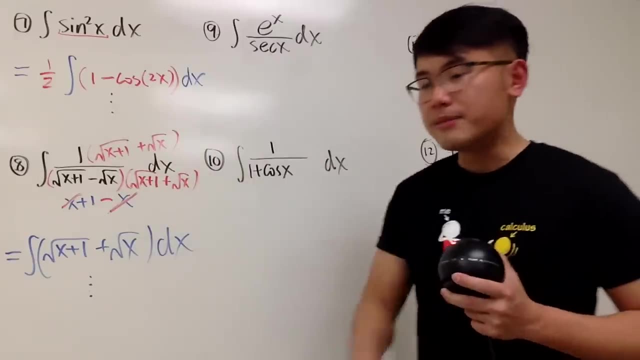 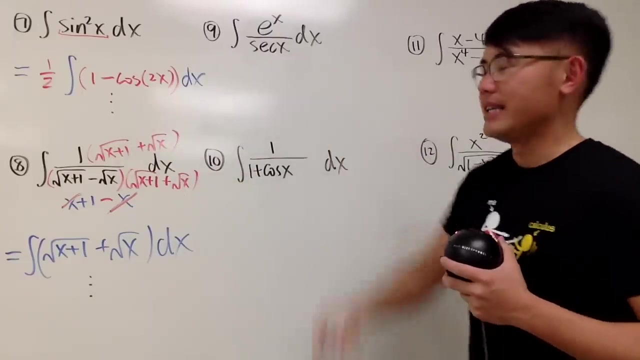 x plus one. you just get du to be dx so you can just go from there. so I put down this for you guys: on the exam do not put down dat, dat. okay, you have to do all the work and then show me the final answer anyway. number 9: 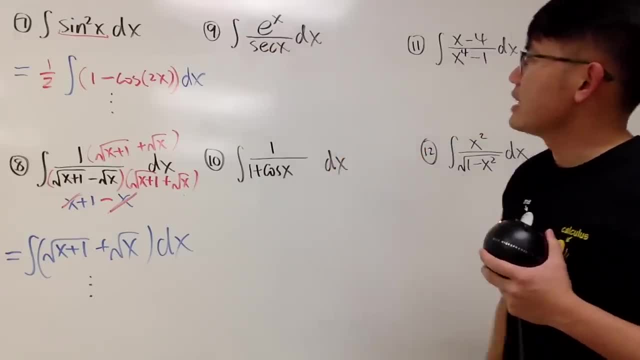 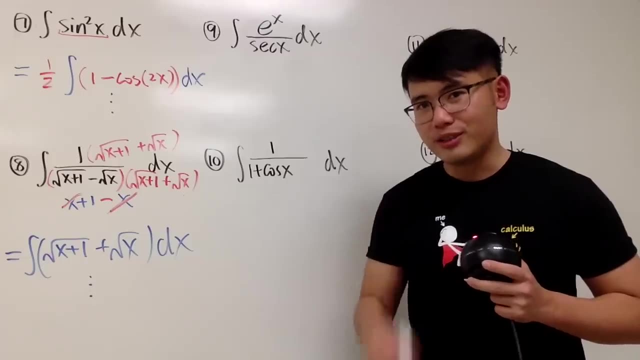 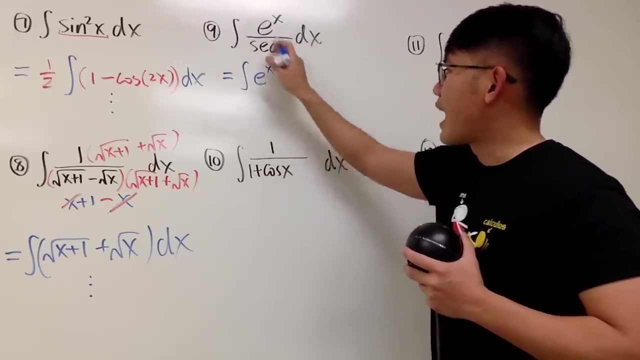 We have e to the x over secant x. But don't forget that secant x in the denominator is the same as what: It's just the same as cosine x. So in fact, this integral is the same as integrating e to the x times cosine x. 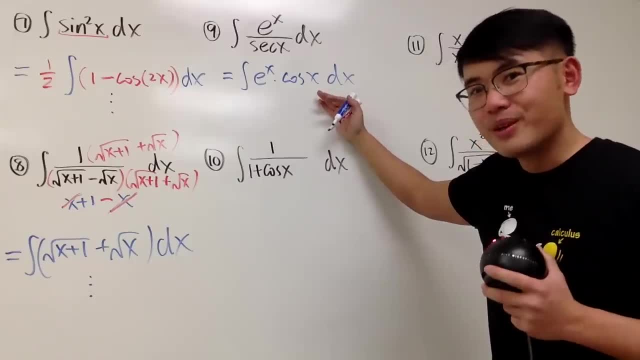 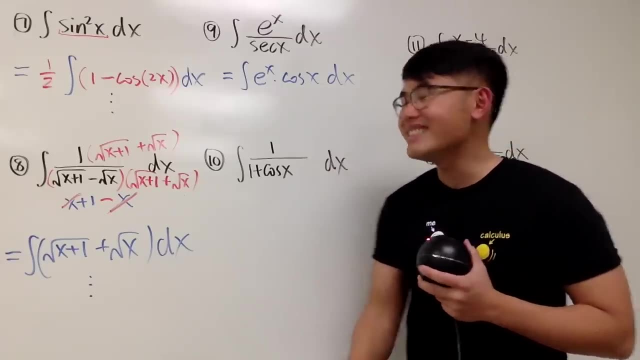 And do we recognize how to integrate this? Sure, we do. How do we do it? Yes, integration by parts, And this, right here, is a famous situation that you are going to get a repeating situation right. So let me just put this down right here for you guys. 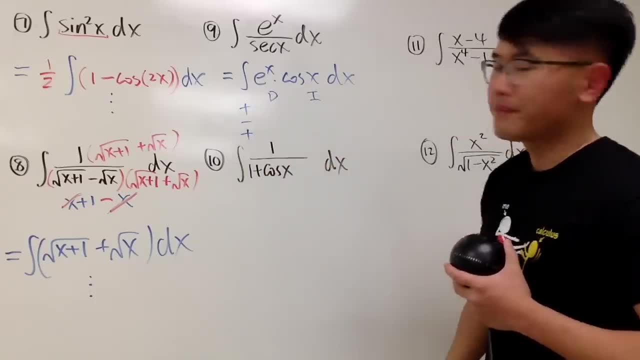 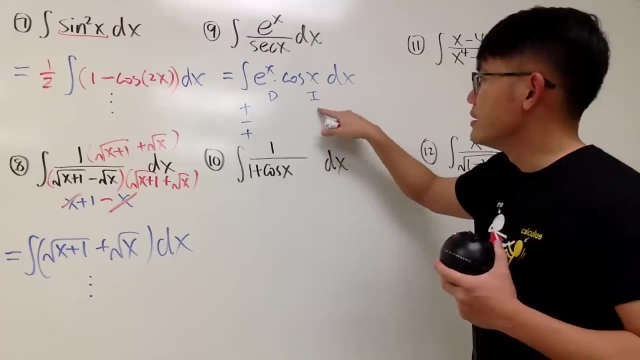 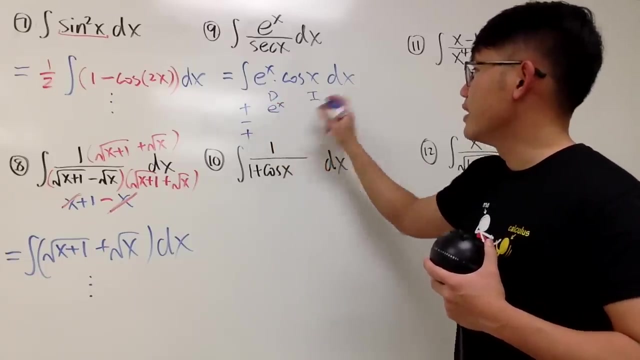 d and i. I need three of them And in fact it doesn't really matter which one you pick to be integrated. They're equally easy. You can integrate cosine. you can integrate e to the x, doesn't matter. But let me just go ahead and differentiate e to the x and then integrate cosine x. 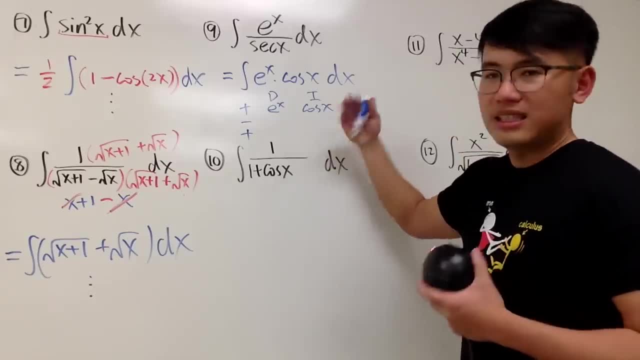 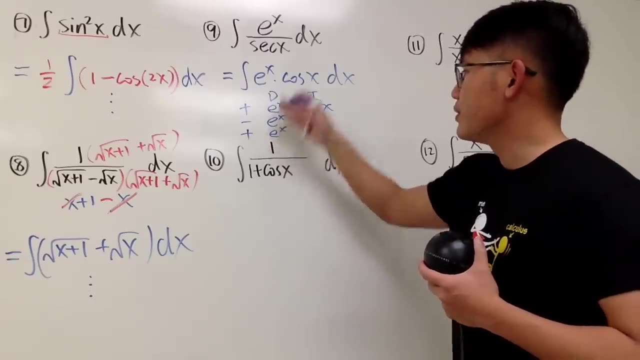 And you may be saying: maybe you want to integrate e to the x, it's easier. That's up to you. This is just as fine. Anyway, you get e to the x, e to the x after you differentiate this. 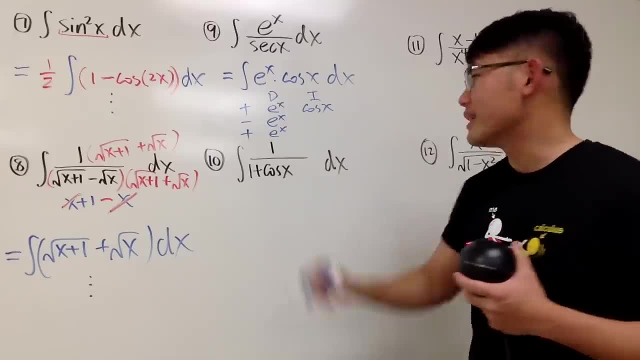 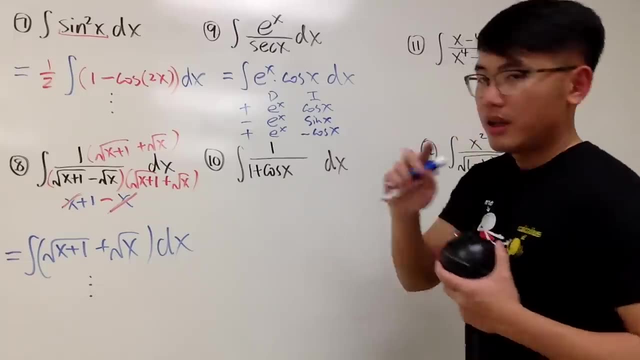 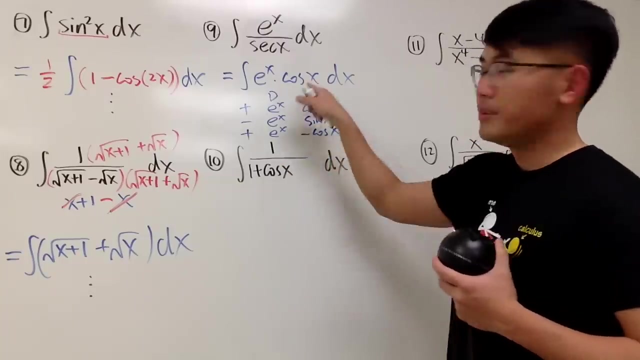 and then integrating cosine x. First you get positive sine x And then integrate this again, you get negative cosine x. Look at the function, part e to the x and then cosine x. This and that repeats right, This, right here, repeat. 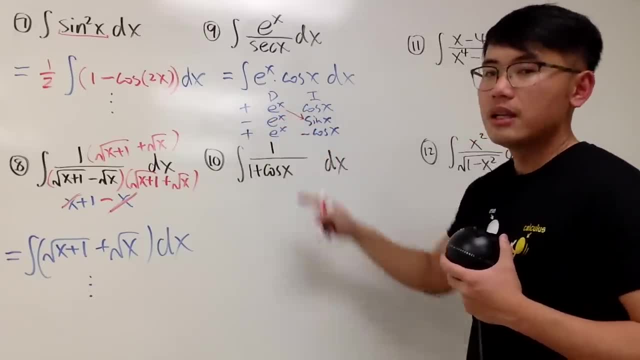 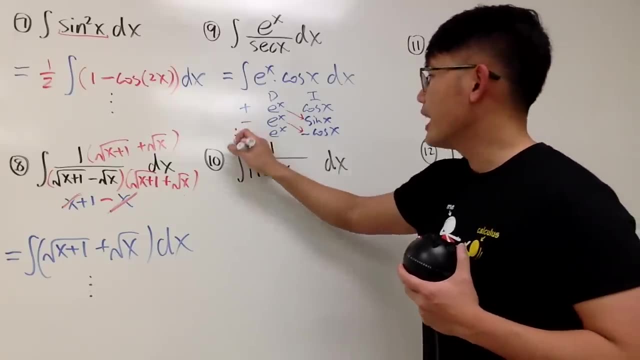 So remember you multiply this and that along with the sine In the front. This is the first part of the answer, And then this, this and that That's the second part of your answer. Don't forget this right here when you multiply. 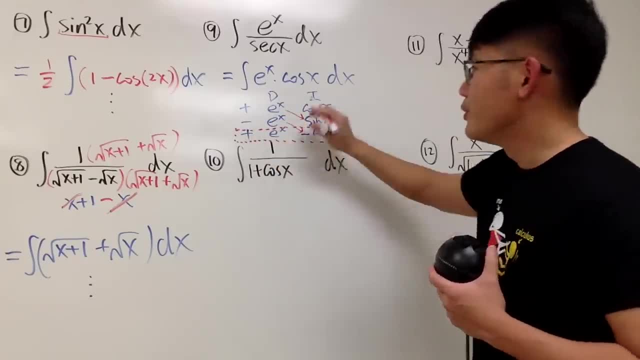 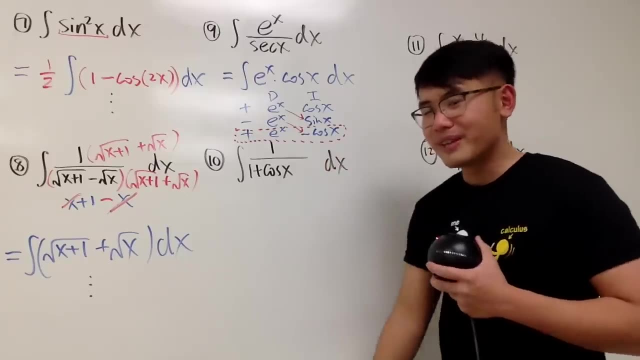 you still have an integral And then you're going to write this down in a line and you will see you have to add this on both sides and you will have to take care of that. It's a repeating situation, right. 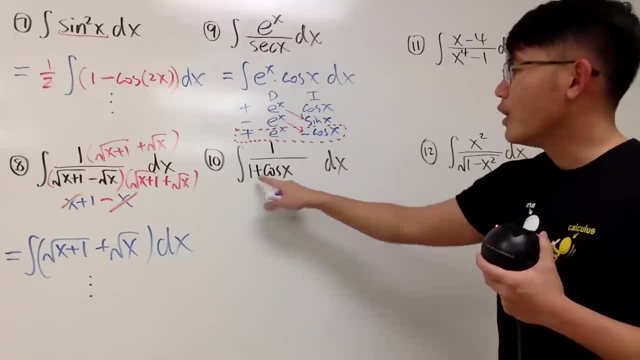 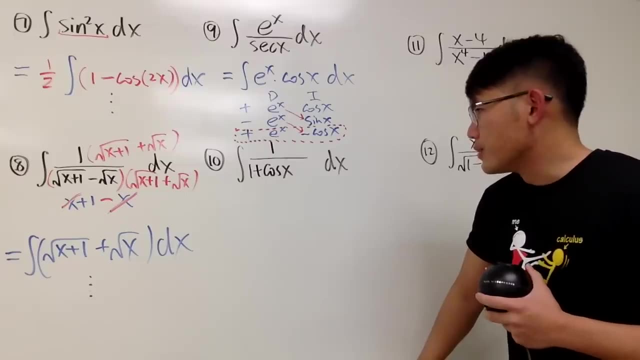 Okay, now let's look at number 10. We have the integral of 1 over 1 plus cosine x. Huh, Again, I don't have sine x. to help me out, What do I do? Well, this right here. I don't like it. 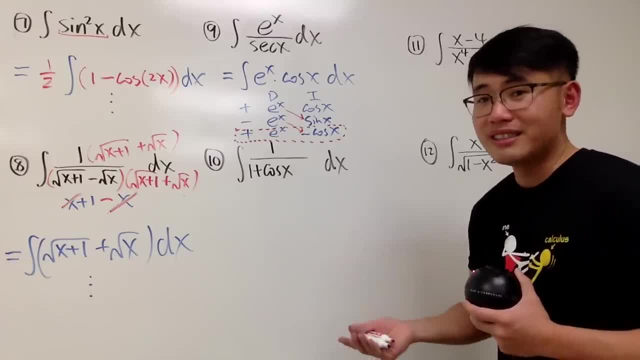 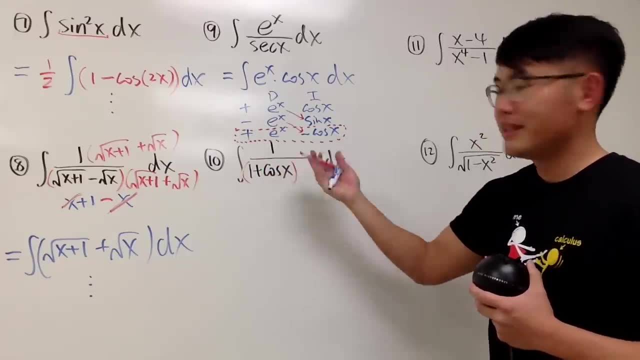 What I like is 1 minus cosine squared, because that's the same as sine squared x, right? Well, it's okay. Let me just go ahead and multiply the bottom and the top by the conjugate. Similar to that. it's going to work out nicely. 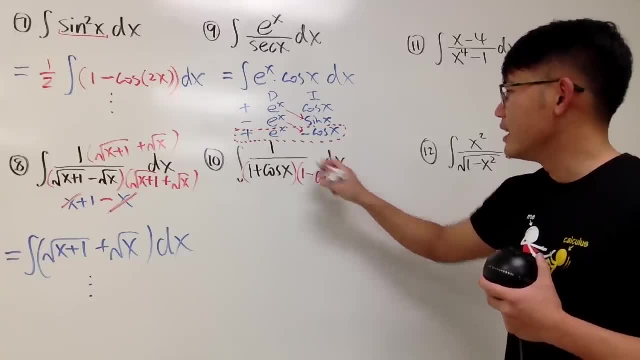 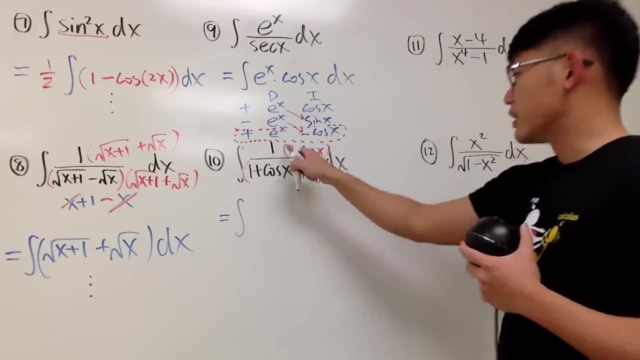 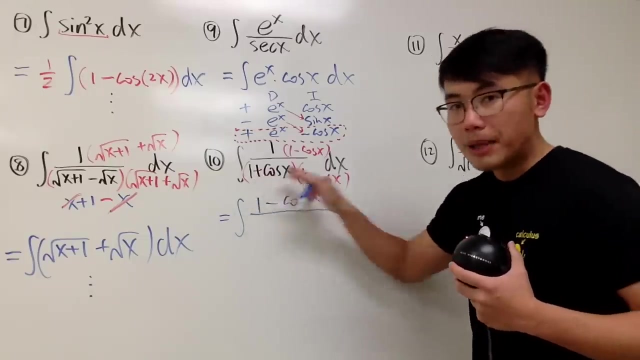 Let's do it like 1 minus cosine x on the bottom and also on the top, And you will see that this is the same as the top is just this, which is 1 minus cosine x, and on the bottom, when you multiply this out, you get 1 minus cosine squared. 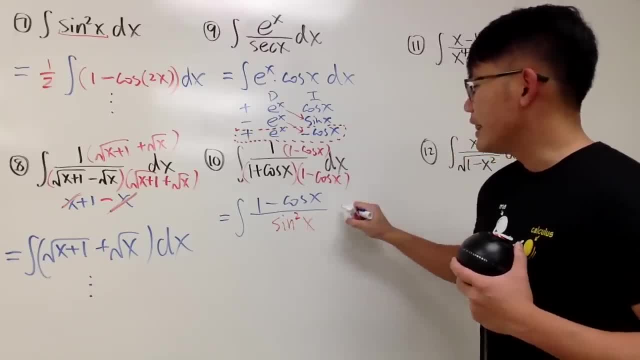 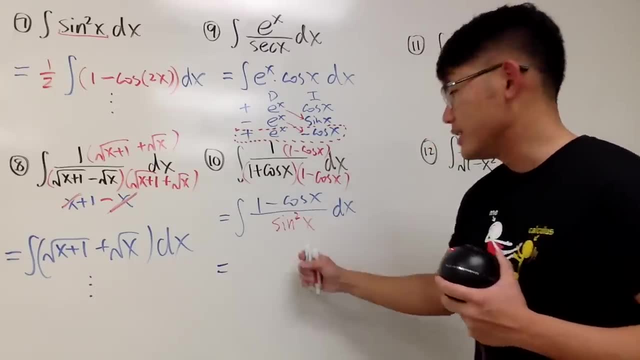 In another word, we get sine squared x, And now we have more things to work with. This is pretty straightforward now, because we can just split the fraction, since we only have one term in the denominator. First integral is the integral of. 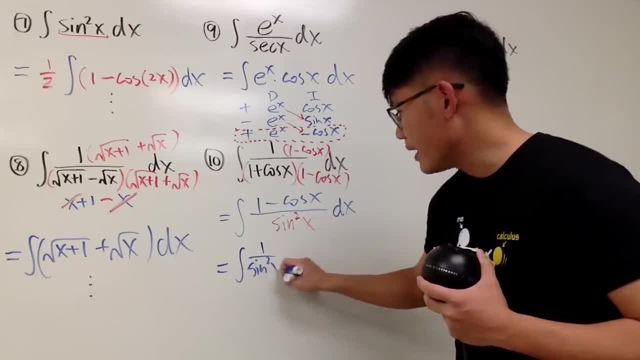 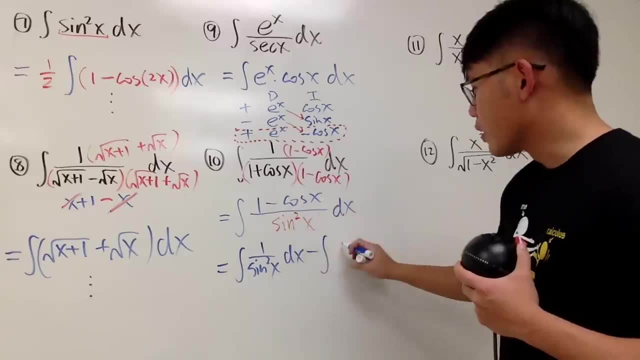 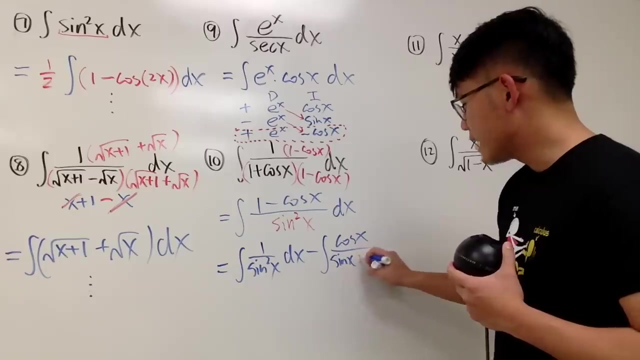 1 over sine squared x, And then perhaps let me close this and then I will put down the minus and then the integral, and then we have the cosine x over sine squared x, And let me write this down as sine x times sine x. 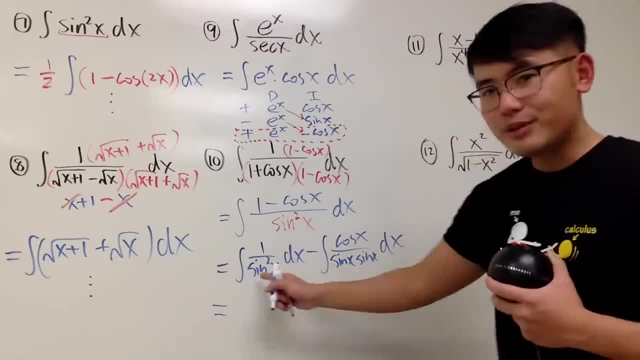 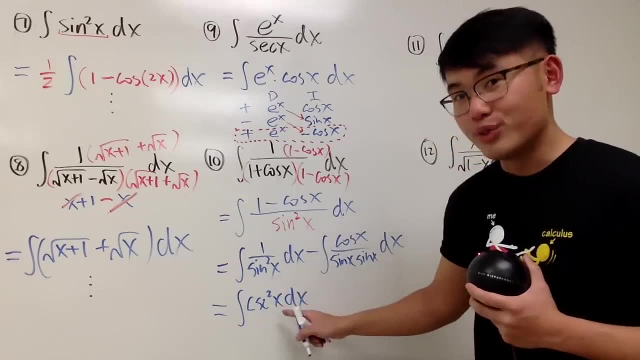 For good purpose. you will see This right here. you just have to focus on integrating cosecant squared x, And you have to know your derivative really well for this So you can write this one right: 1 over sine is cosecant. 1 over sine squared is this: 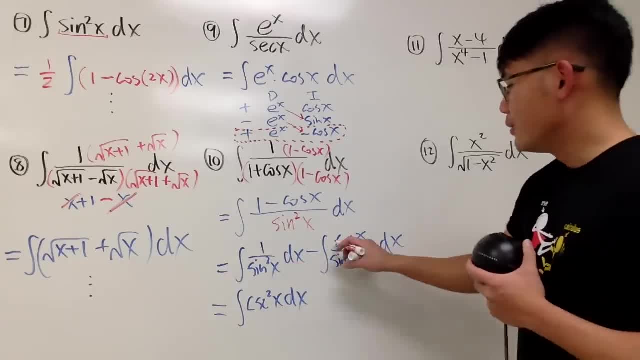 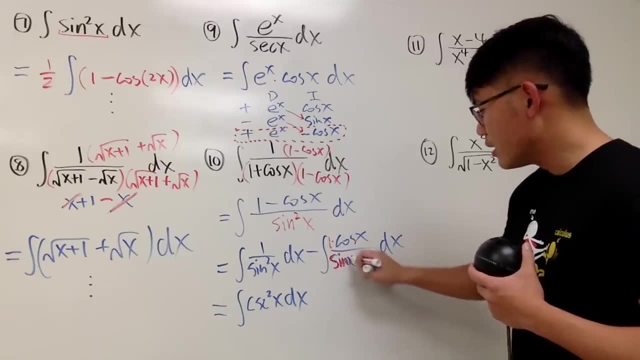 So in fact this is pretty easy now. But for this one, look at, I have this over that. This is like saying 1 times cosine over sine x. So you can say this is minus the integral 1 over sine is cosecant x. 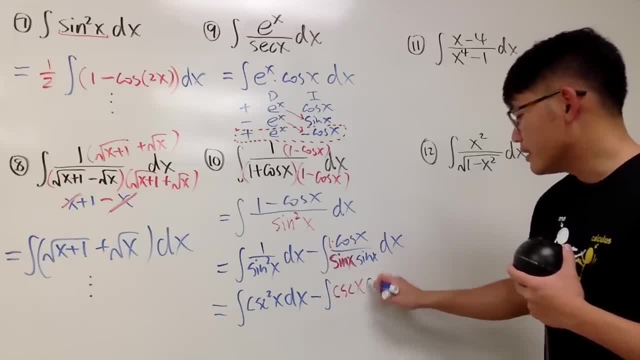 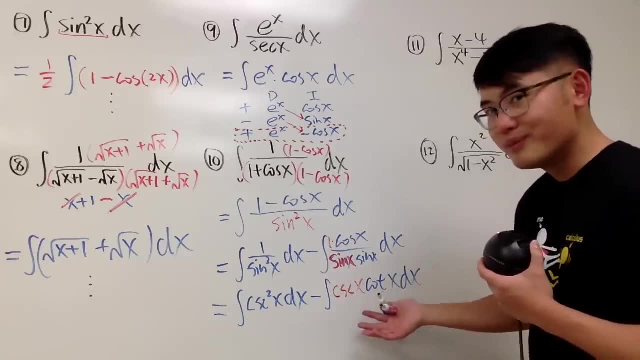 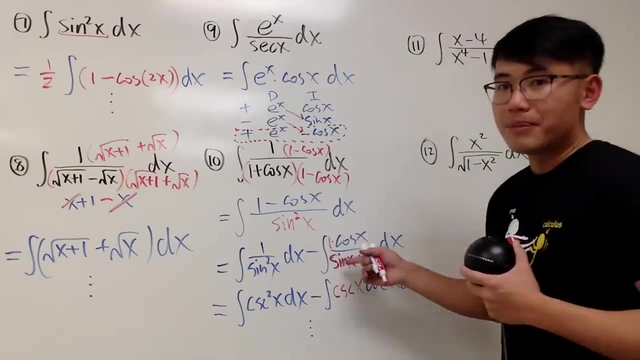 and then cosine x over sine x is cotangent x, dx. And again, if you recognize this is the derivative of some function, then you can integrate that. But again I will leave this to you guys, Or right here you could have done, use up as well. 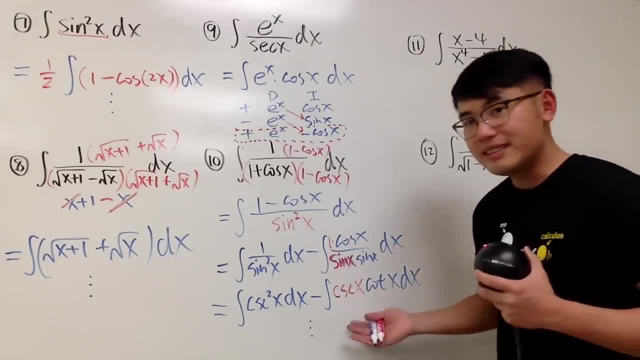 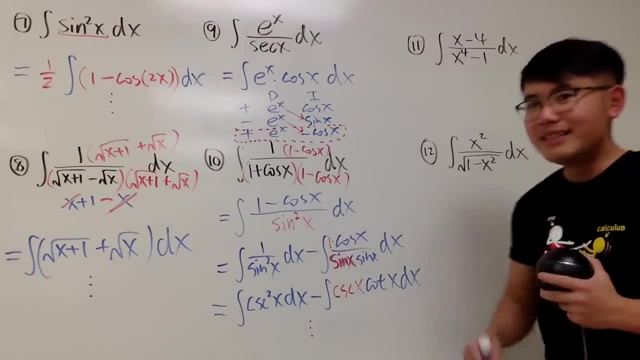 That's fine. But once you put this down in this form, you can just recognize this by knowing the derivative of some function is equal to this, which is very nice. Okay, two more right, And once again, let me know if you guys like this or not. 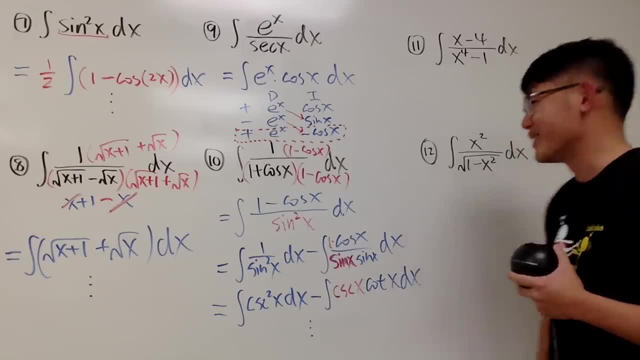 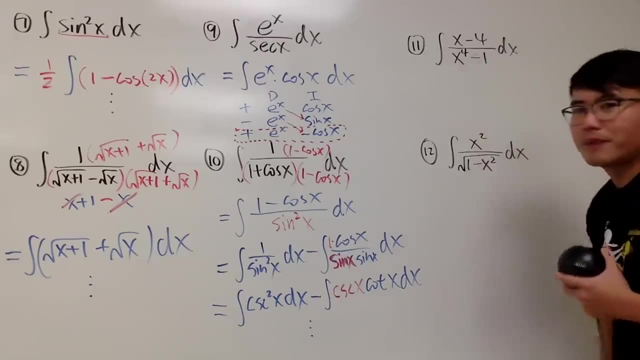 If you guys do, maybe I'll produce part two like the other ones for you guys. Okay, number 11.. x minus 4 over x to the fourth, power minus 1.. The derivative of the bottom. it's not the same as the top. 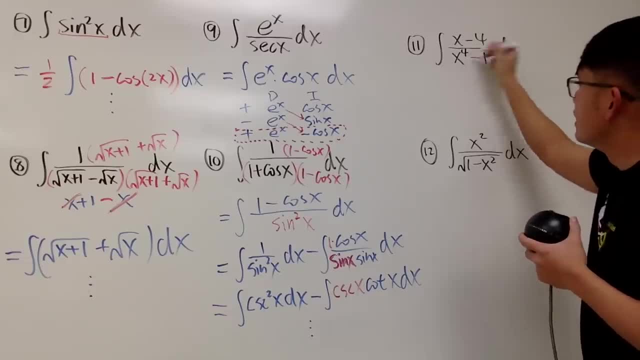 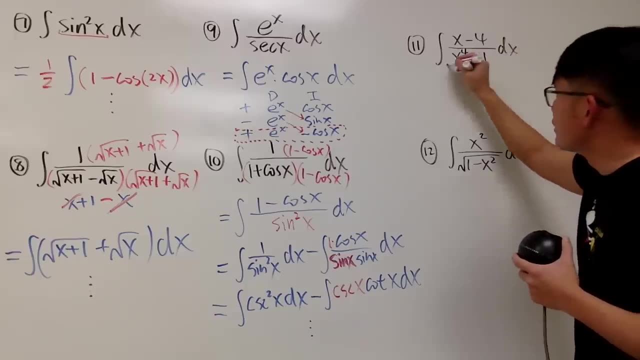 Partial fractions, then right. So let's factor the denominator This right here. look at this as the difference of two squares: first x squared squared minus 1 squared. So first you can factor this as x squared minus 1 times x squared plus 1.. 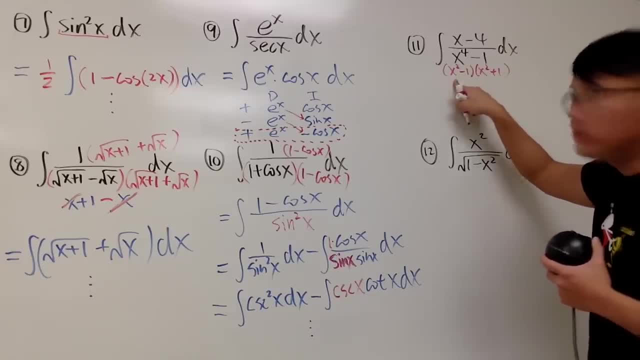 All right, And then this is still factorial. You can factor this to be x minus 1 times x plus 1.. But this is no longer factorial. You keep it. This is an irreducible quadratic, All right. And then the general form for this situation is that: 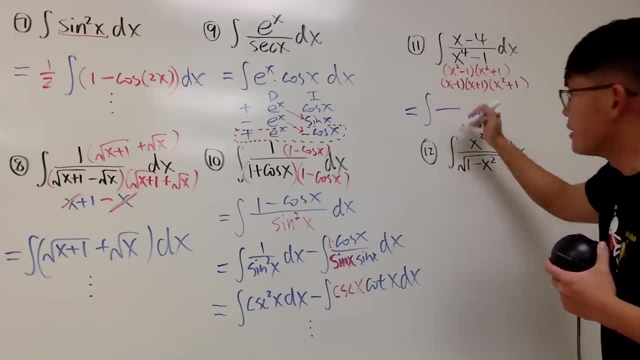 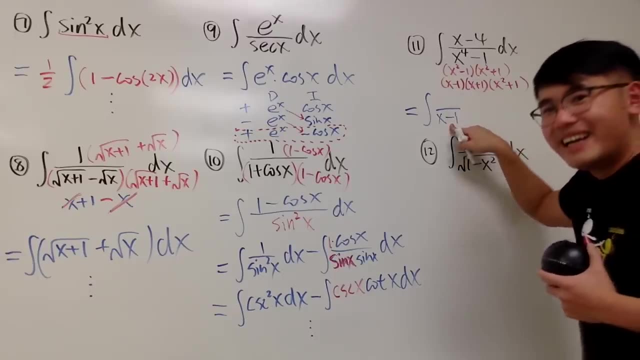 well, first of all, you have this for its denominator, So I'll put down x plus 1.. Well, the first one I put down is negative, so I'll put a minus here. Anyway, this is the linear. That means the top has to be just a constant. 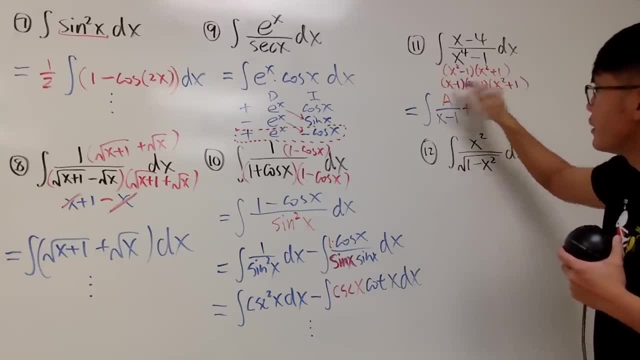 And then next I have another linear factor. This is different than that. So I put down x plus 1 and it has to be a constant. on the top. Next one, we have x squared plus 1.. This is an irreducible quadratic. 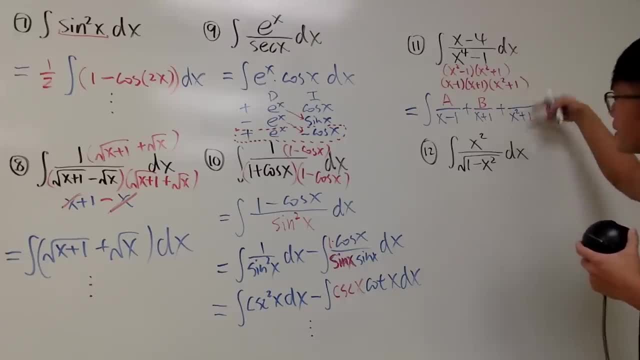 So I will write down x squared plus 1, but the top has to be one degree less than this, Namely it has to be a linear now. So I will put down cx plus 1.. So that's d, a, b, c, d, all that. 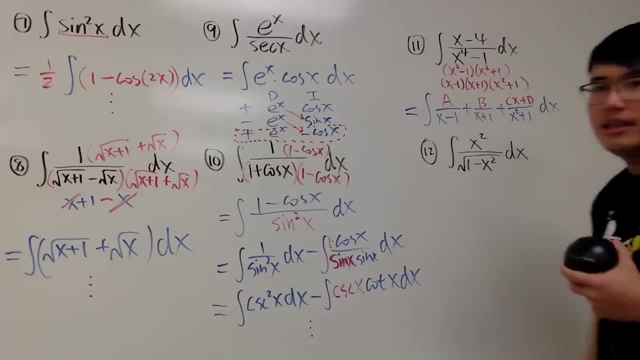 And then, of course, you're going to find out the a, b, c, d and then integrate them, right, So I'll leave that to you guys. Okay, For this one right here, don't erase the x squared on the top and just say: 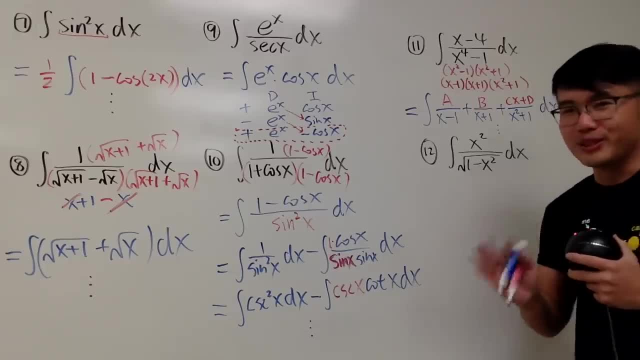 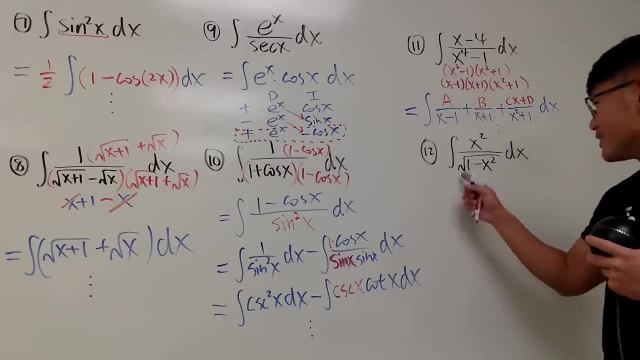 hey, I want to have the x on the top. That would be so easy. You can just do it yourself for this situation, right? But you do have to handle this x squared Here. we have square root, So I'm going to write down square root. 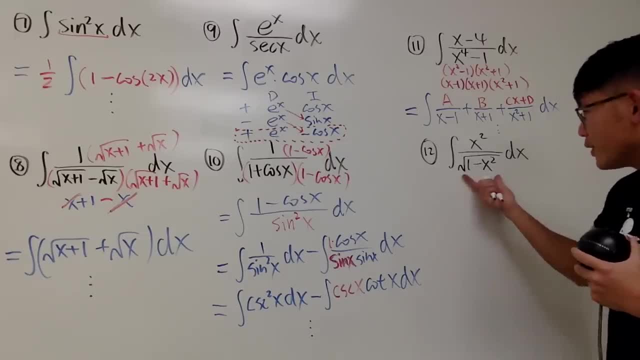 So I'm going to write down square root. So this is not a partial fraction situation And technically this is just one term, the square root term, So you don't do the conjugate like that. Well, in the square root we have 1 minus x squared. 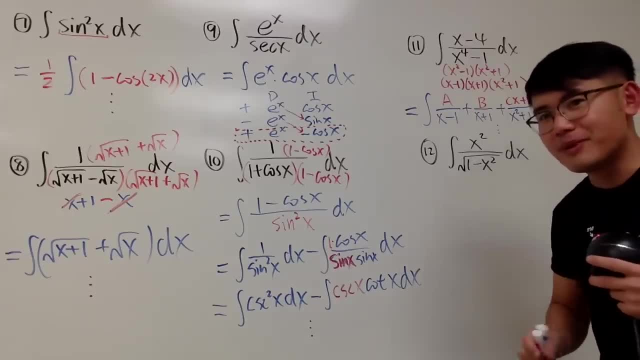 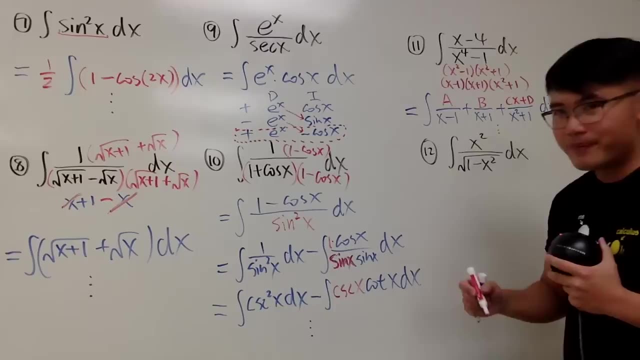 It has two terms. Yes, we can do tricks up for this, And we have to know that 1 minus sine squared will give us cosine squared. You can also use this 1 minus cosine squared to be sine squared, but you know, just take. 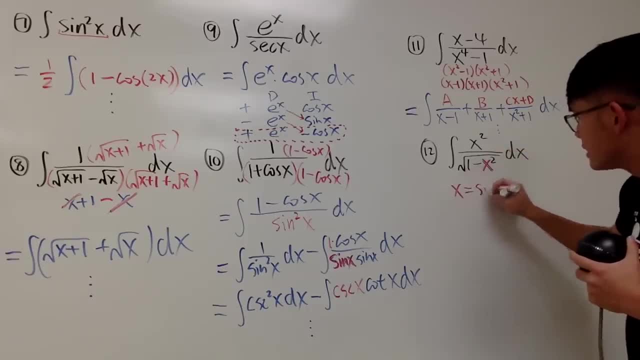 take this x to be sine theta, right, Of course you have to change that to the theta world. So let x equal to sine theta. That's the deal. And then don't forget to change the dx, So I will have to differentiate this on both sides. 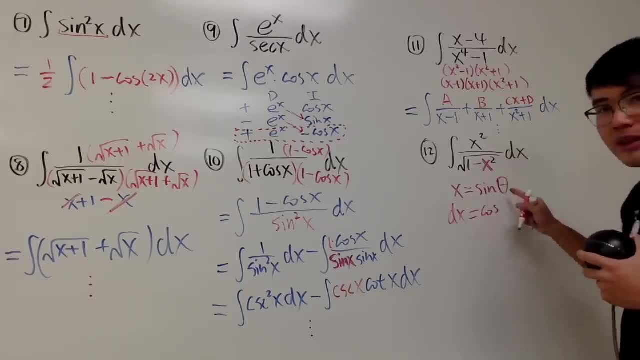 So I will get dx to be the derivative of sine theta. You are doing the derivative right here. okay, Now integral. So from here to here it's just the derivative. You get cosine theta, d theta And that's pretty much it. 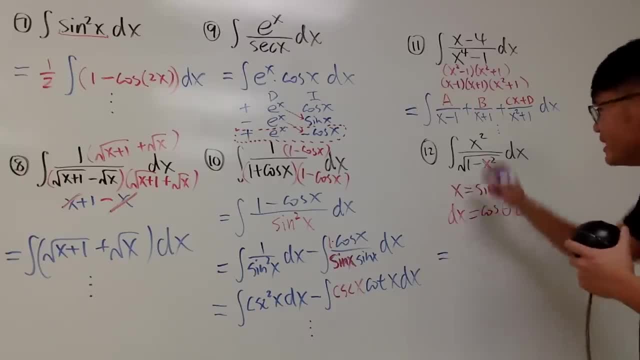 But I think I will work this out for you guys to have some more space. Why not? Here we have the integral On the top. I have sine right, That's x, And then you square that, so we have sine squared theta. 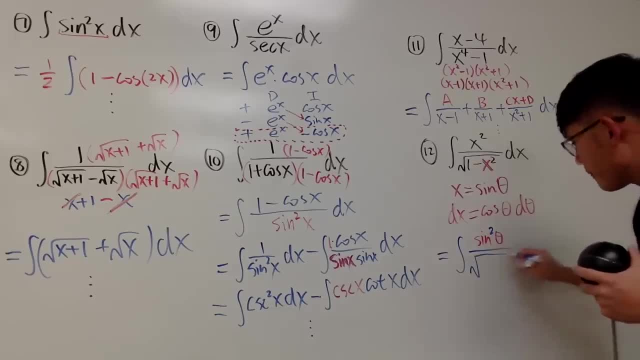 On the bottom here we have square root And then we have 1 minus sine squared again, So we have sine squared theta. So here is a super common mistake. People don't like to put down a, d, whatever This right here. if you don't put down anything, 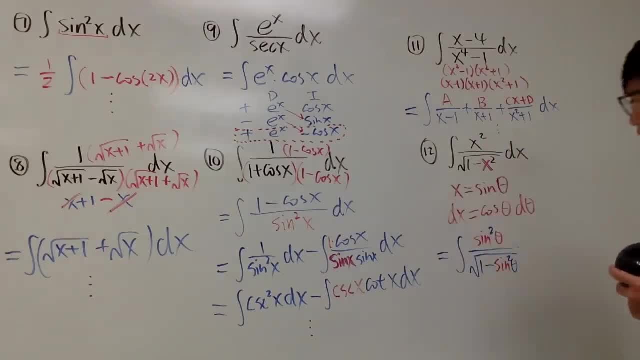 that's like driving without your seat belt on- Very dangerous, So don't do that. Remember, dx? you did the hard work, So put it down. This right. here is cosine theta d theta. okay, And now we'll clean things up. 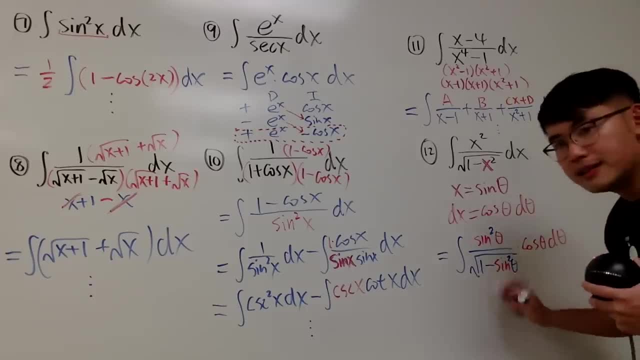 Right here in the denominator. I'll just focus on this square root part. This cosine squared theta by the square root. After you cancel the square and the square root, don't worry about the absolute value, Just focus on cosine theta, because you just